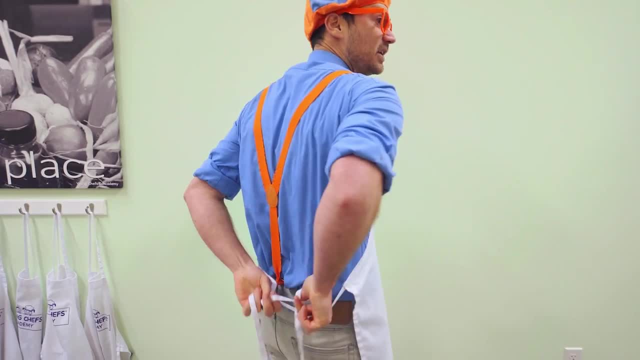 Yeah, an apron is used, so then clothes not get dirty when you're cooking. Okay, now we're going to rinse our hands. Okay, now we're going to rinse our hands. Okay, now we're going to rinse our hands. 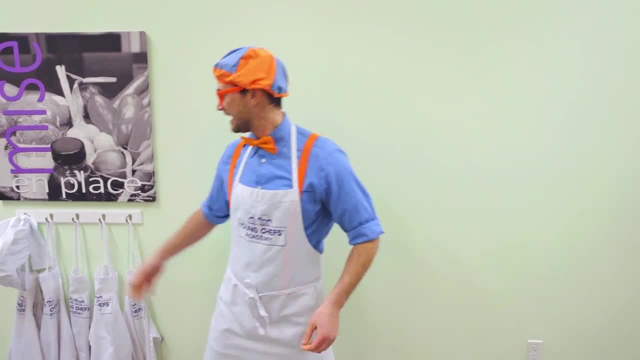 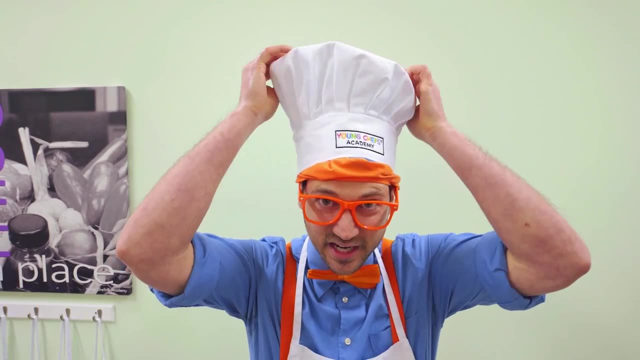 With some food, With some food, All right. And can't forget my young chef's academy chef's hat, chef's hat, How do I look? How do I look? All right, Check it out, Check it out. 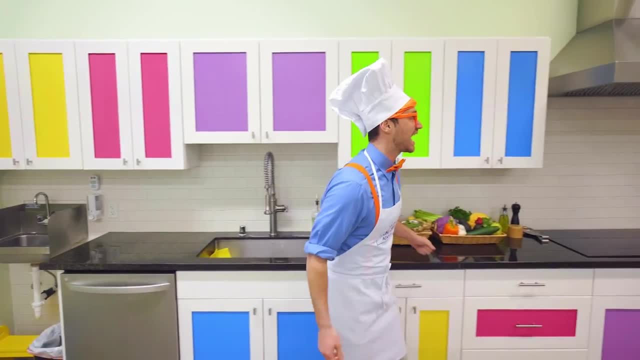 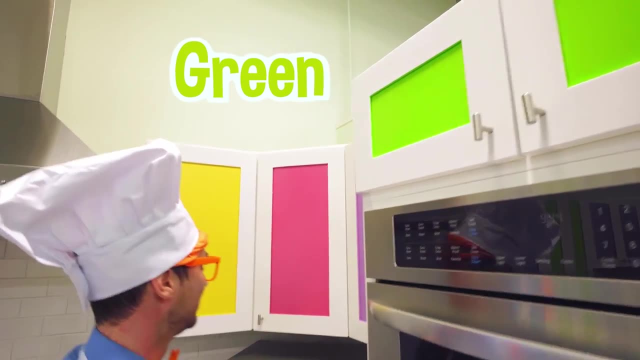 This kitchen is so colorful. Do you see all these cabinets? Yeah, Do you see all these cabinets? Yeah, Whoa, These, yeah, are the color green. These, yeah, are the color green. Ooh, Ooh. 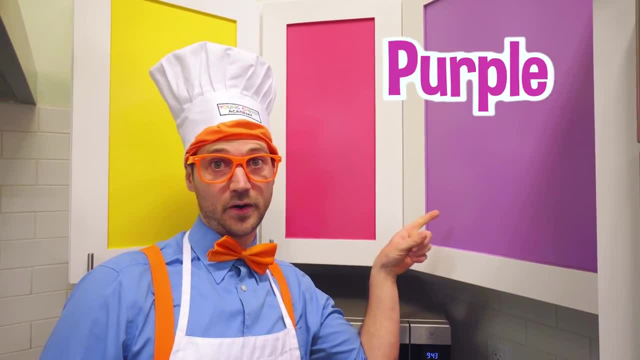 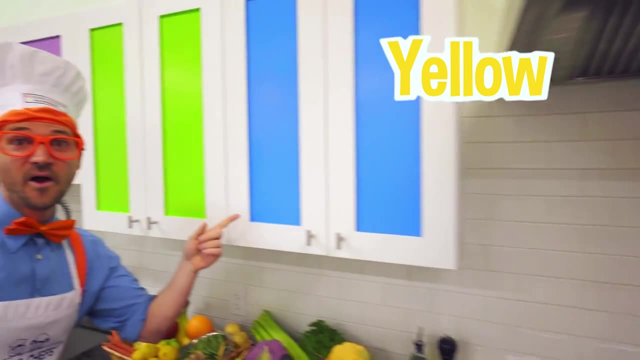 And this over here, Yeah, And this over here. that cabinet is. that cabinet is purple, purple, pink, pink, yellow, yellow and blue and blue and blue, Whoa Whoa. I bet there's a lot of cool things in these cabinets. 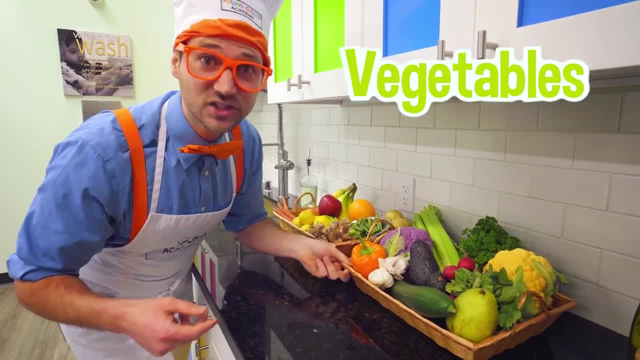 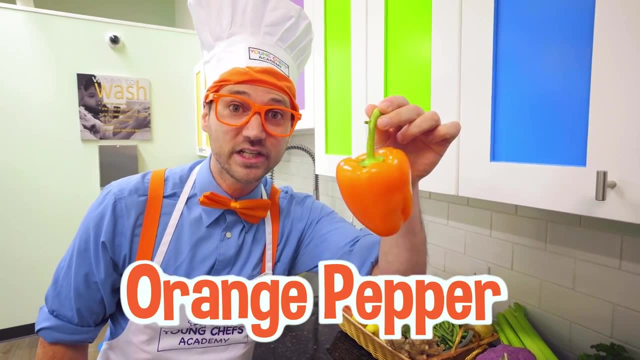 Whoa, Whoa. Look at this. Look at this. Some yummy vegetables. Some yummy vegetables. Hey, Hey, Do you know what kind of vegetable this is? Yeah, Yeah, This is an orange pepper. Look at these. yeah, some green beans. 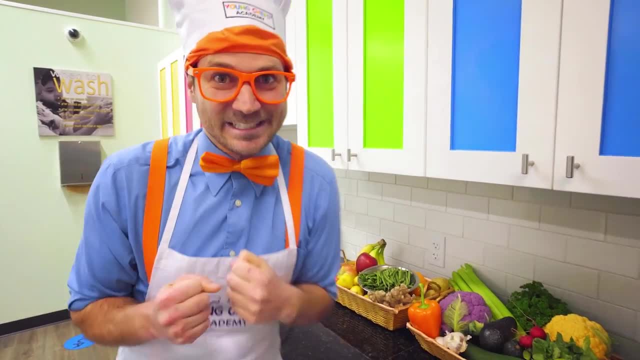 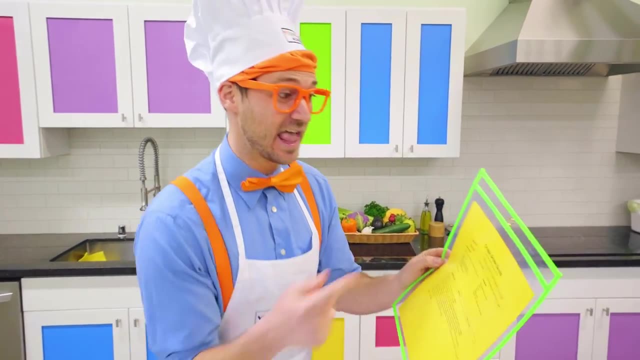 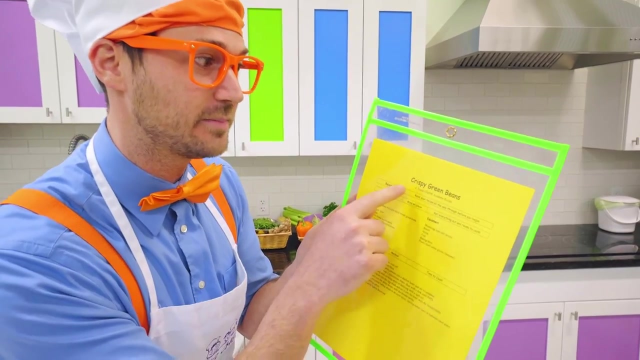 I sure do love vegetables. All right, I'm so excited. Whoa, I am so excited. This is gonna be tasty. I am looking at the recipe of what we're gonna be making today. Looks like we're gonna be making crispy green beans. 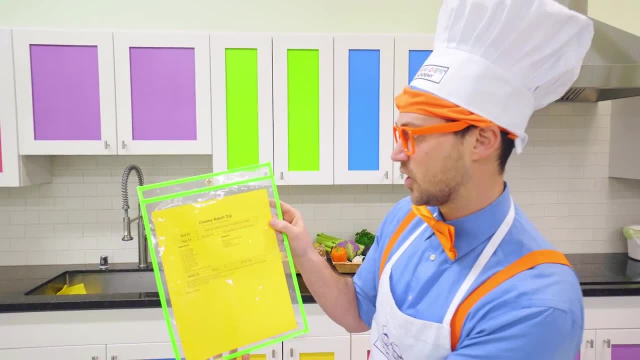 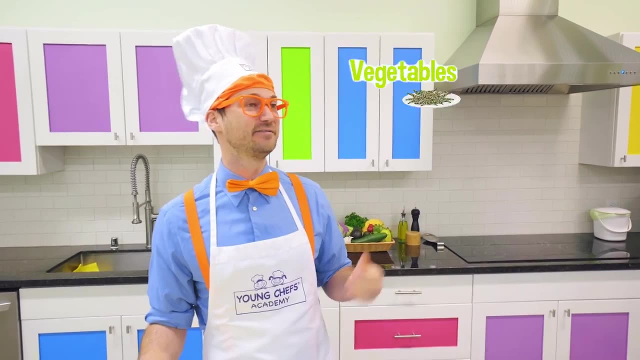 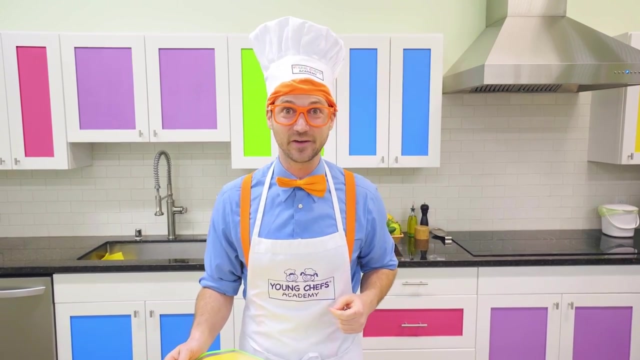 Whoa, those look tasty And creamy. ranch dip- Oh, this is gonna be so yummy and healthy. I love vegetables and I love ranch dip. I wonder if we're gonna be able to dip the green beans into the ranch dip. Yeah, 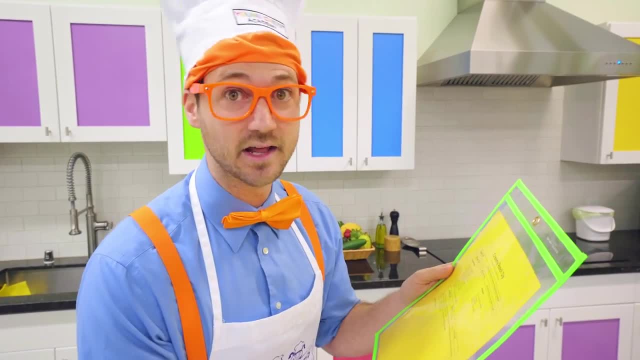 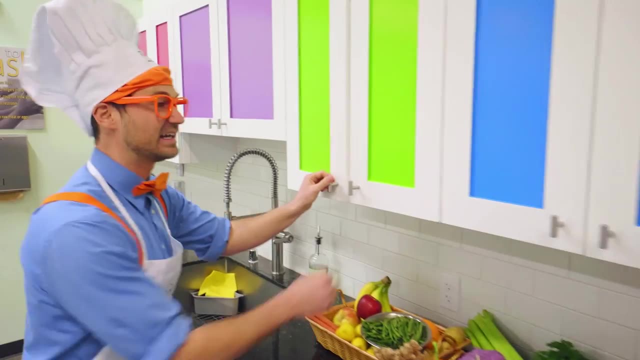 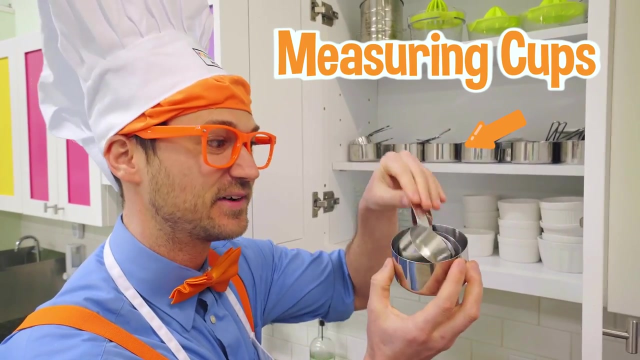 Okay, so it seems like we need a lot of tools and a lot of ingredients, So let's get to it. All right, let's see what's in here that we need. Okay, looks like we need some measuring cups. Oh, a small one. 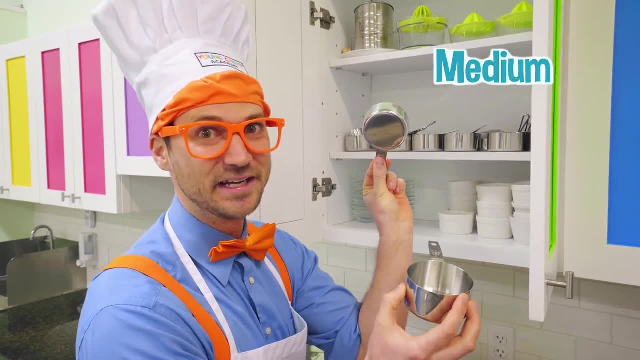 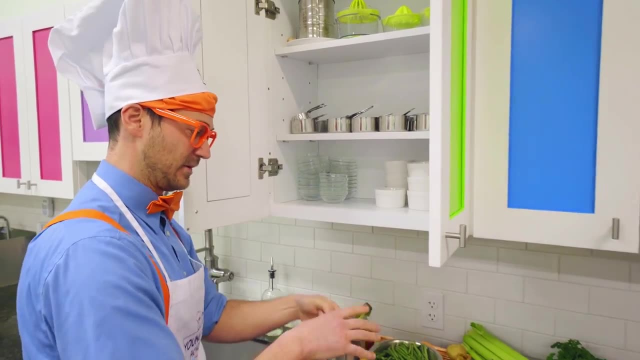 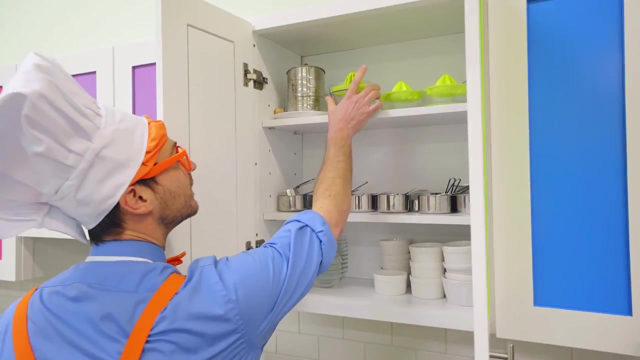 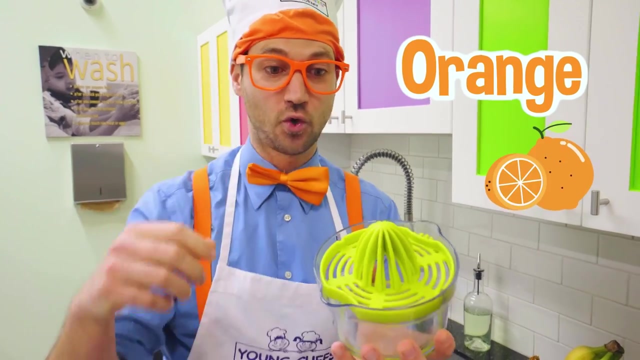 A medium-sized one, Another medium-sized one And a big one. Okay, Put those right back here. Perfect. Then we need whoa, a juicer. This is where you can put a lemon or an orange or a lime. 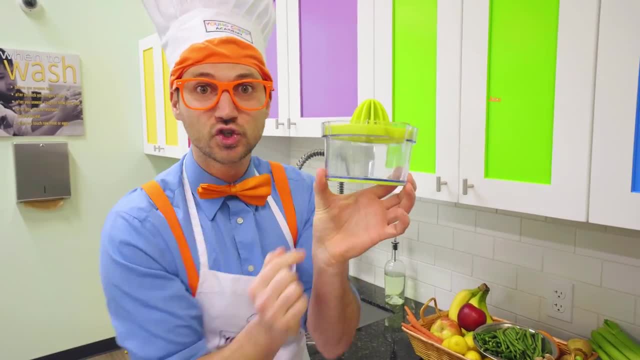 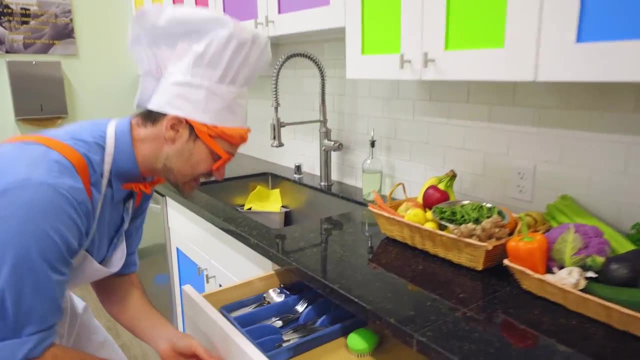 Squeeze it on top and then all the juice comes out the bottom. Okay, we'll set that down right there. All righty, let's see what's in here. Hmm, oh, we definitely need some measuring spoons, Whoa. 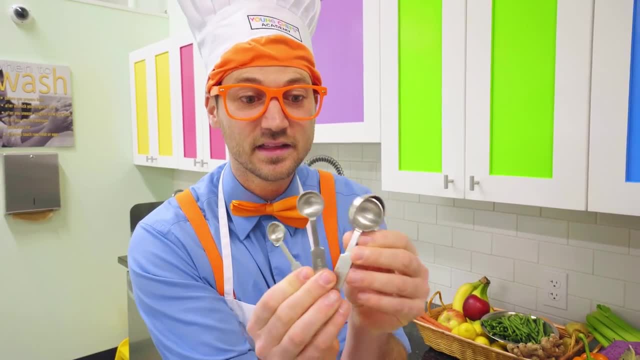 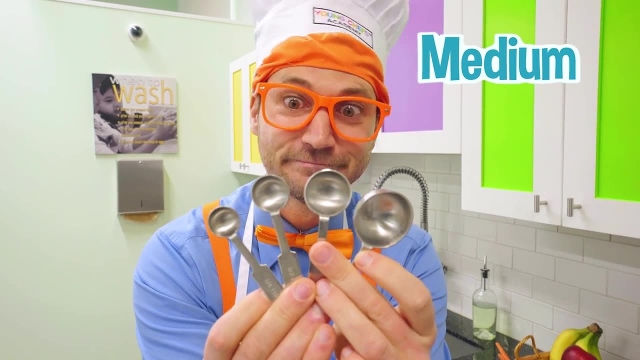 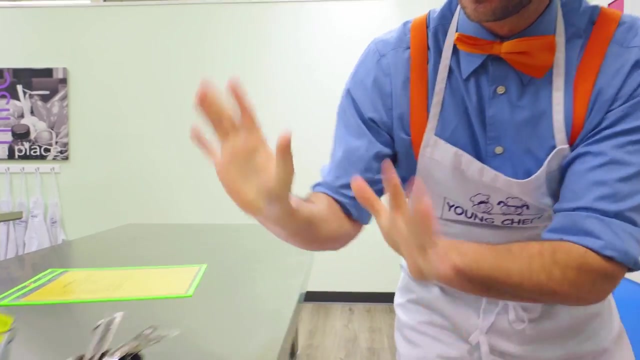 Yeah, same thing, just like the measuring cups, Measuring spoons of four different sizes, From small to medium To medium to medium to large. Okay, put them right about right in there. Perfect, Okay, let's see how about? oh wow, a measuring cup. 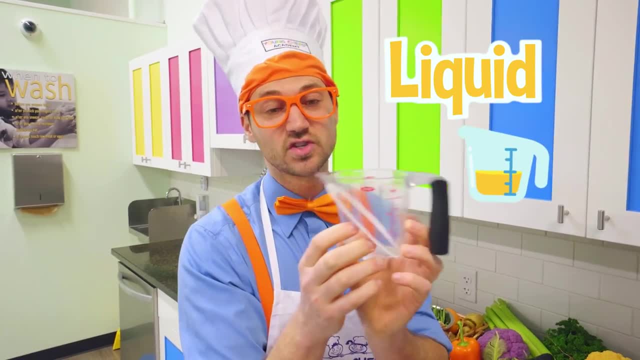 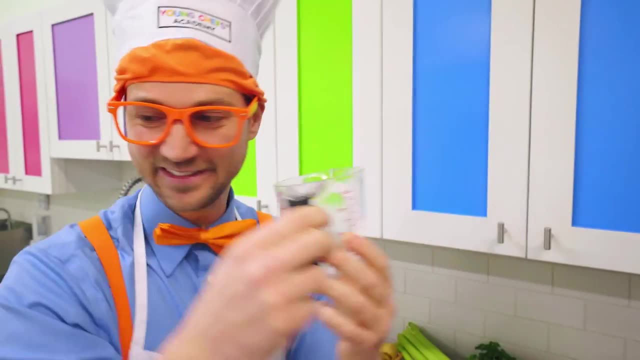 This is what you put: liquids- and you could do solids, but this is primarily for liquids, And this is what you measure to see how much you have. Okay, put that down right there. Oh, let's see, Is there anything in here? 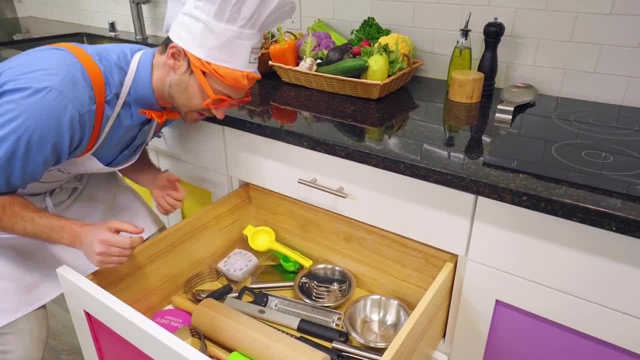 Hmm, there's a lot of cool things in here. Whoa. look at this, It's a rolling pin. Oh, so cute. This is a small rolling pin, Whoa. And this is a big rolling pin, Whoa. 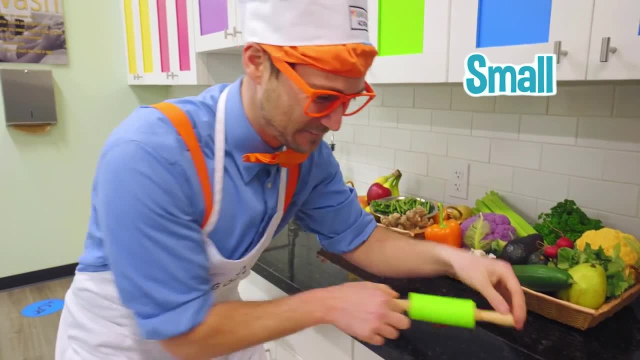 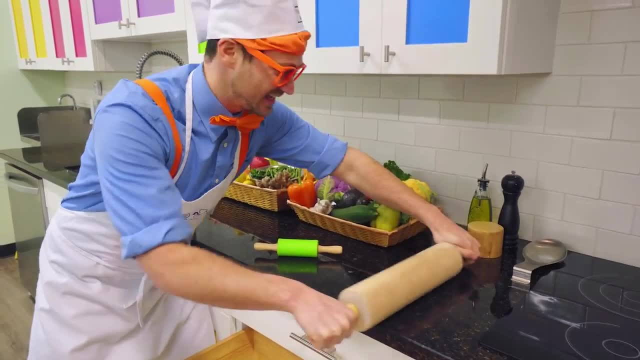 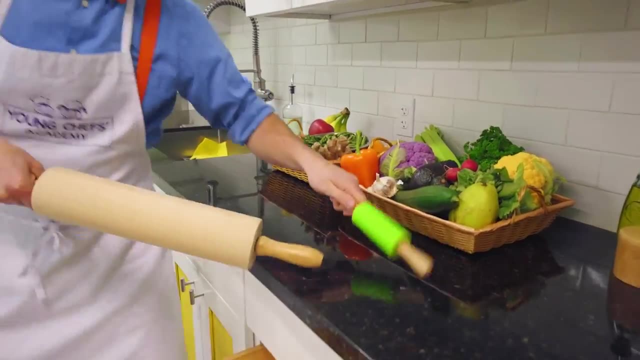 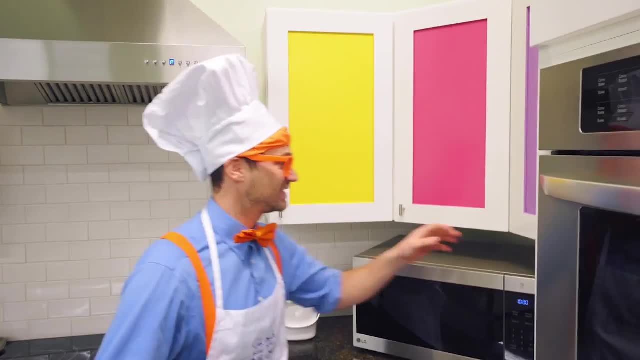 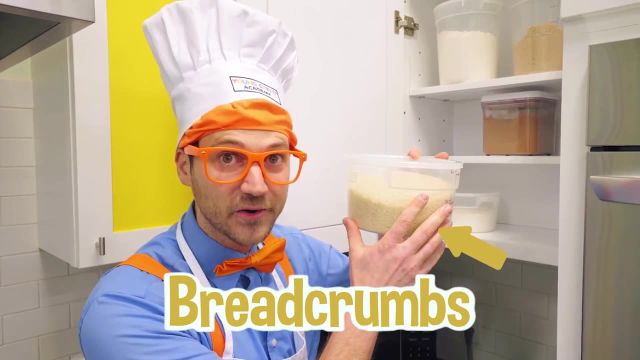 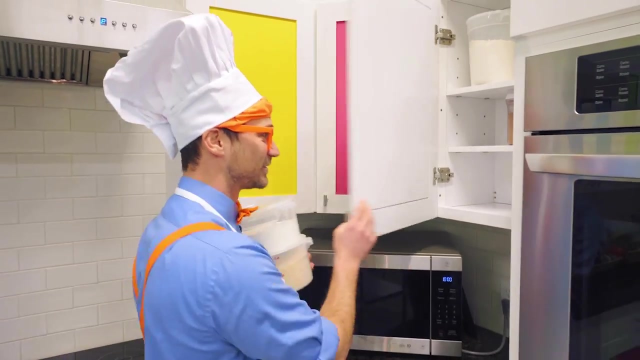 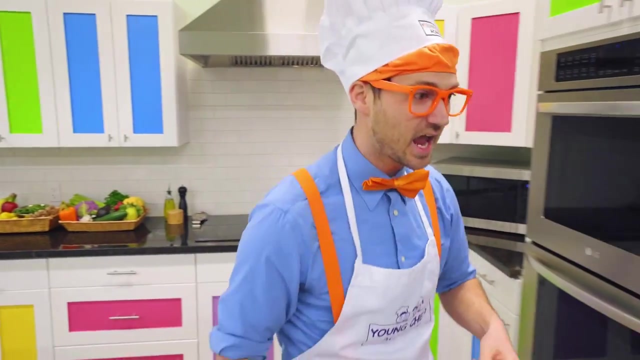 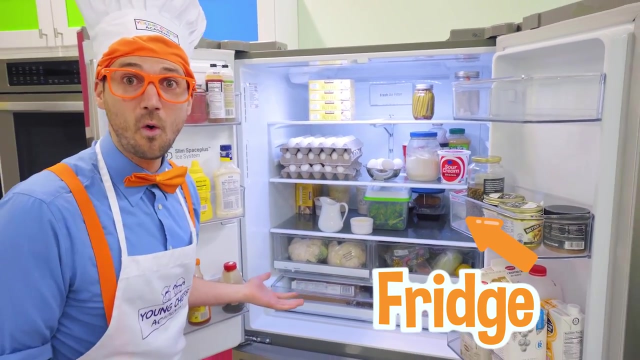 All right, let's see. Probably right in here. Oh yeah, Two ingredients that we need: Breadcrumbs and flour. Perfect, We'll shut this. Great, there we go. Let's see how about some cold ingredients? wow, look at this fridge. it's so organized, okay, looks like. 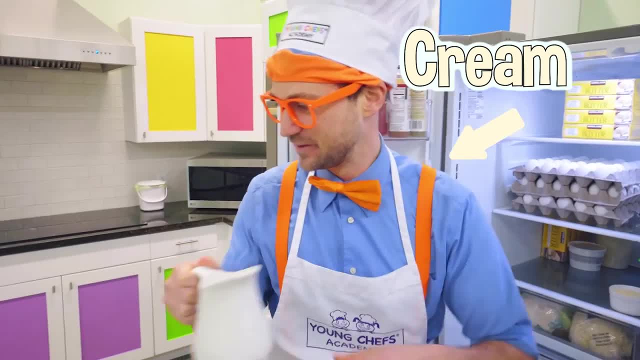 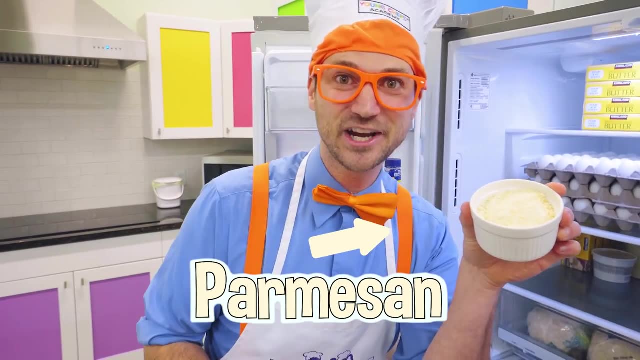 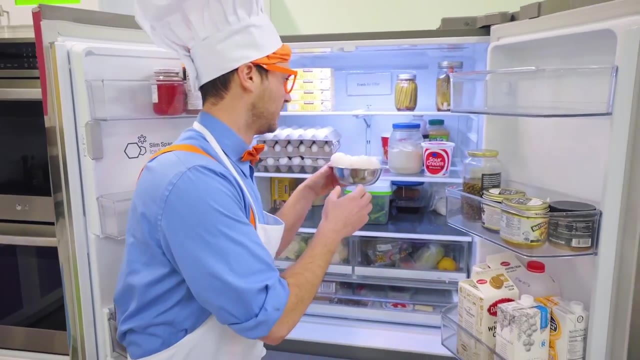 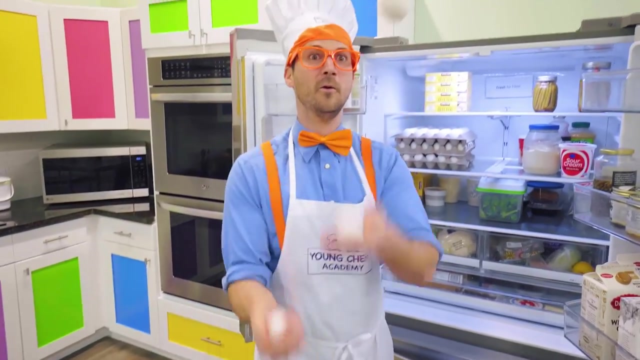 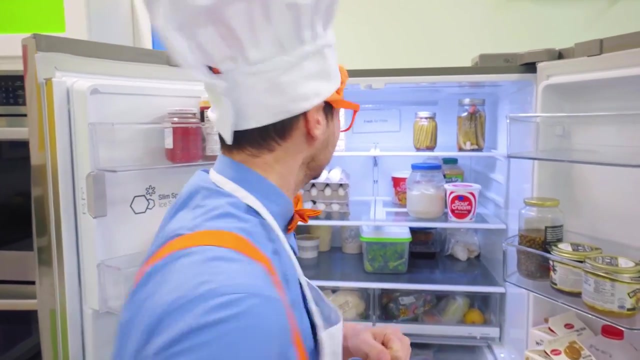 we have some cream, probably for the ranch dip. we'll set that down right there. oh, some cheese- parmesan cheese- okay, we'll put that down right there. and then we have some eggs- yeah, check this out- whoa. okay, put those down right there for later. probably shouldn't do that at home. and then we 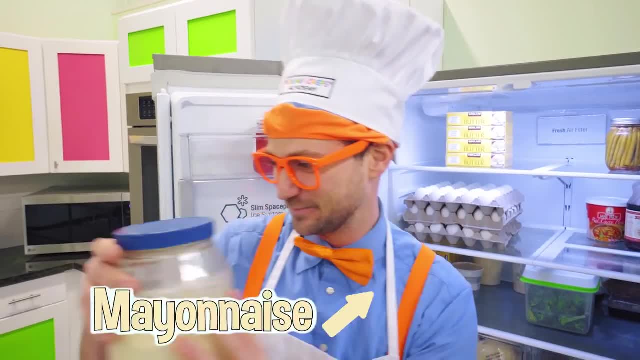 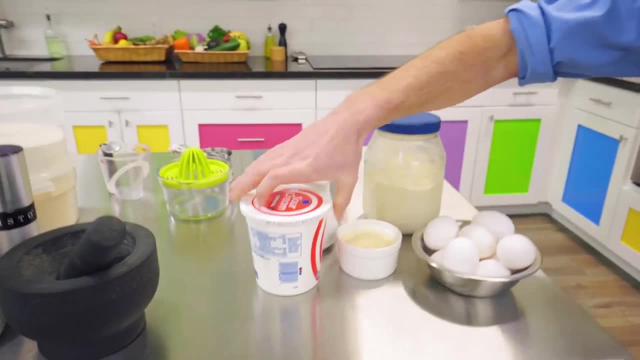 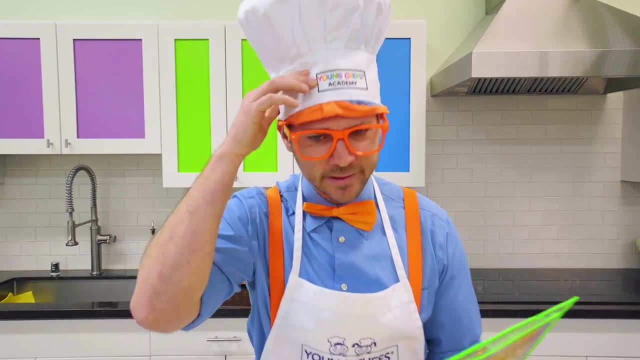 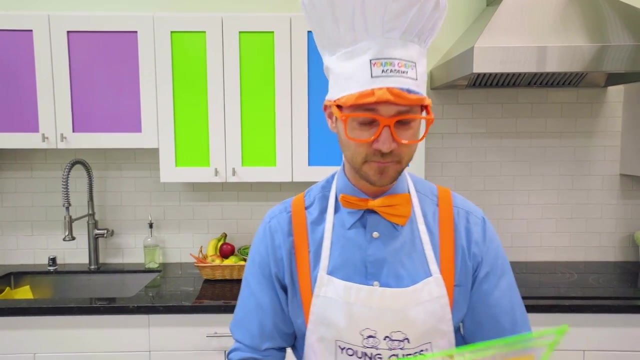 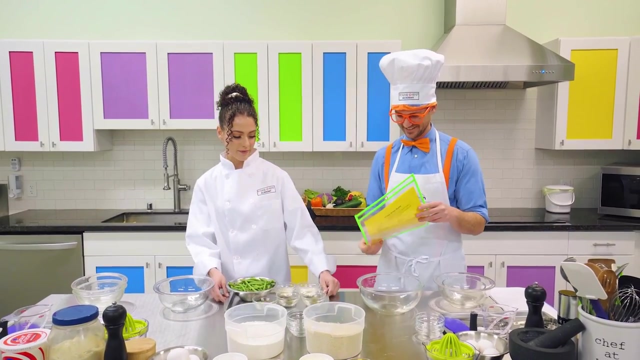 have some mayonnaise- put that down right here, and some sour cream- okay, put that down, and now i think we're ready. looks like we have most of the ingredients and tools, but this looks really hard. oh no, if only i had some help. huh, want some help with these. oh sure, hey, hi, i brought the 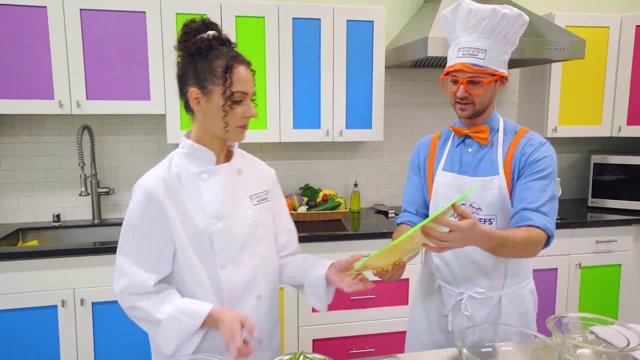 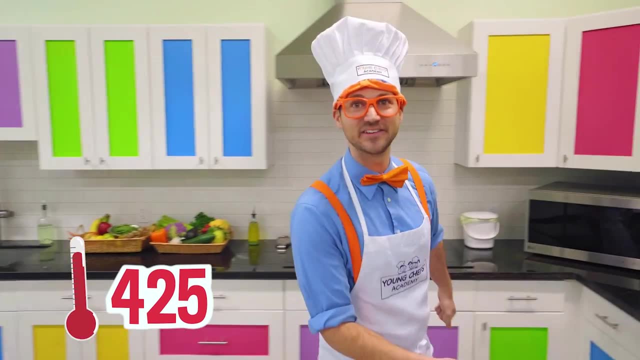 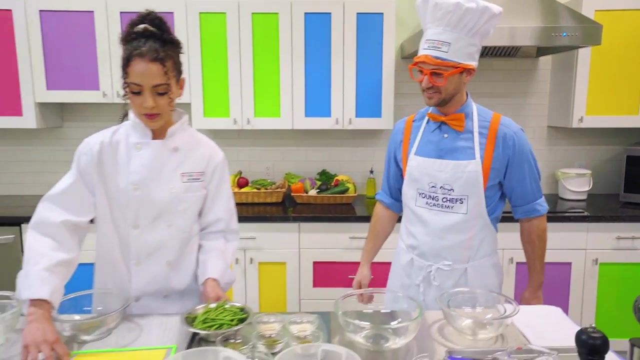 rest of our ingredients that we need. oh, perfect, okay. well, here's the recipe. what do we do first? first, we're going to want to preheat the oven to 425.. okay, uh, i know how to do that. okay, preheat the oven to 425.. perfect, good job. thank you all right. first we're going to want to do a tablespoon. 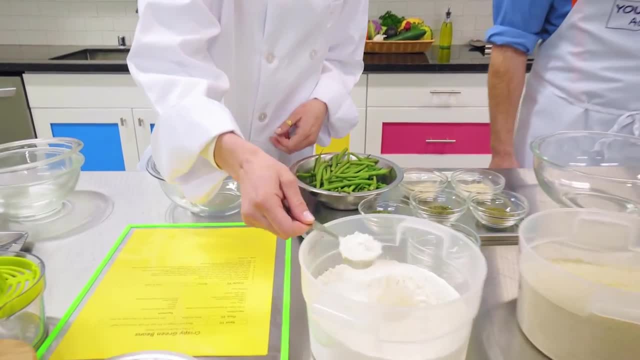 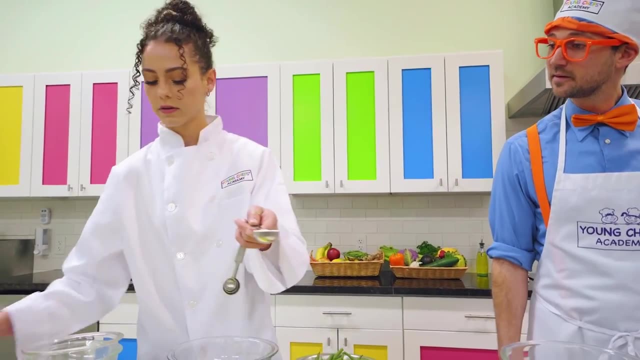 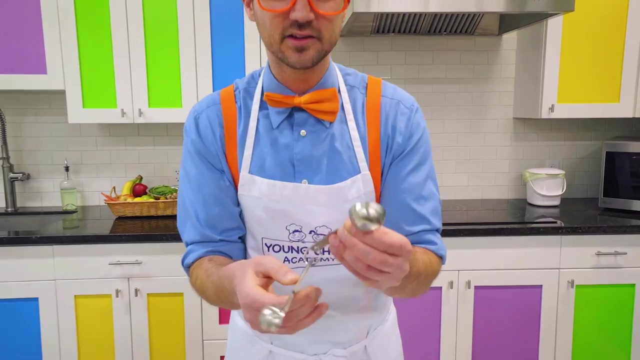 of flour into our bowl. okay, we're going to want to make sure that we get a true tablespoon, because that is not accurate. so we want to scrape off the extra flour. okay, okay, can you do that, sure? okay, looks like we need some flour. let's do a little scoop. 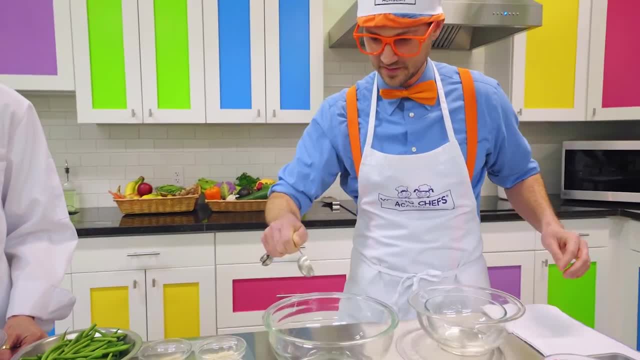 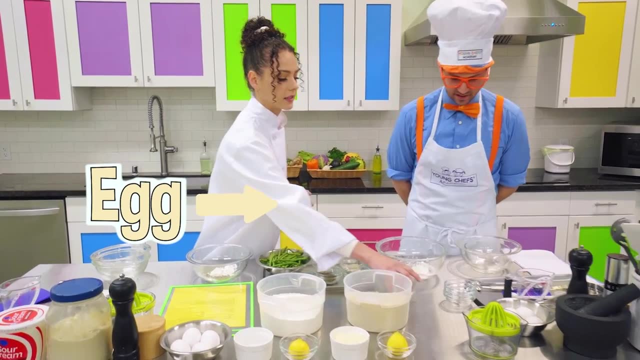 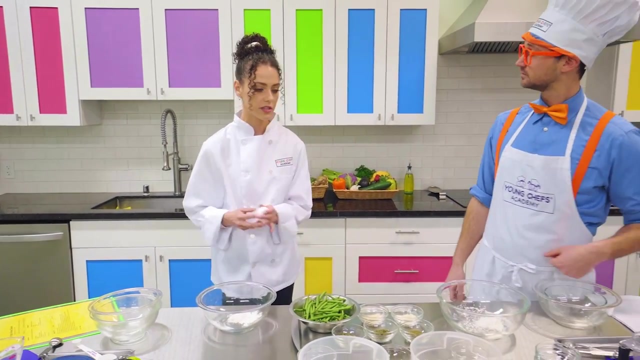 and there we go and perfect. great job, loopy. all right. next we're going to want to crack an egg. okay, so at young chefs academy we crack an egg using the table, not the edge of the counter, so that it doesn't get all over the floor in the mess. okay, you want to crack hard. 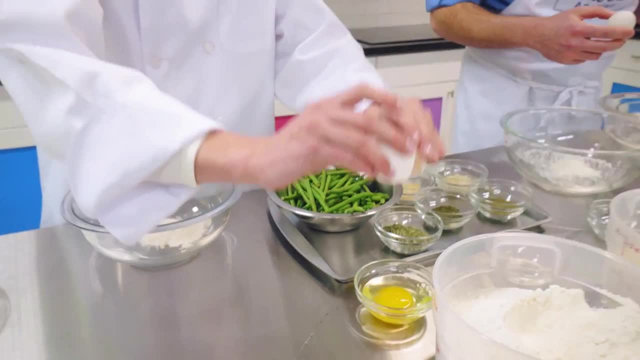 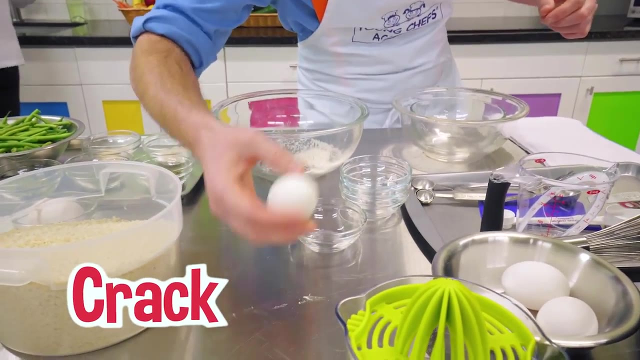 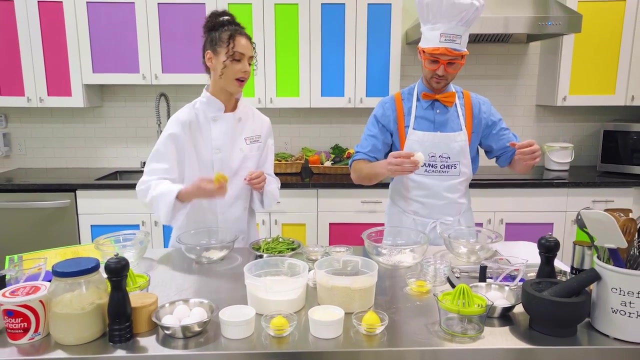 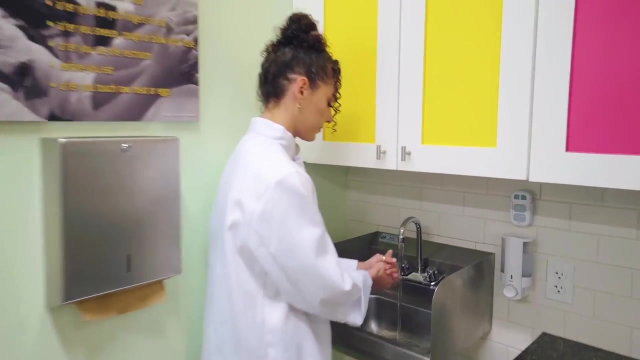 and use your thumbs to break open the egg, just like that. perfect. i don't want to break the egg, the shell, in a separate bowl. okay, here we go. let's use the table. there we go. great job, thank you. we're gonna wash our hands because we touched a raw egg. 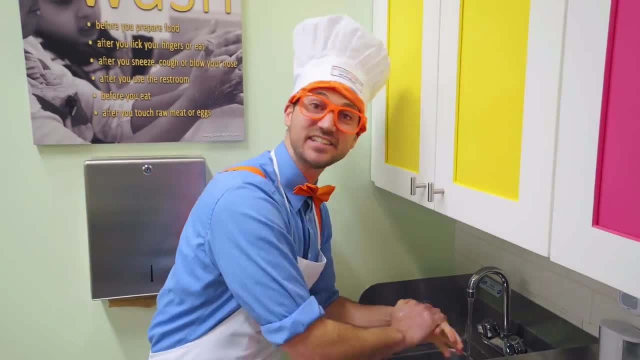 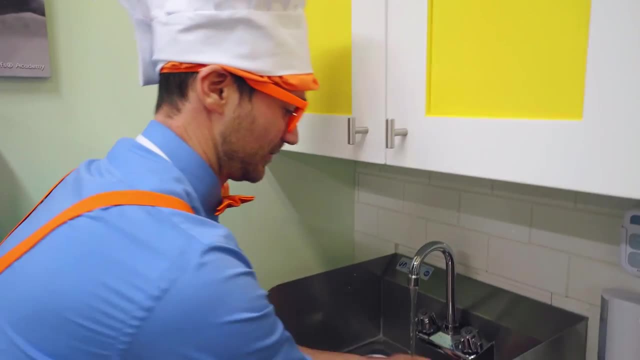 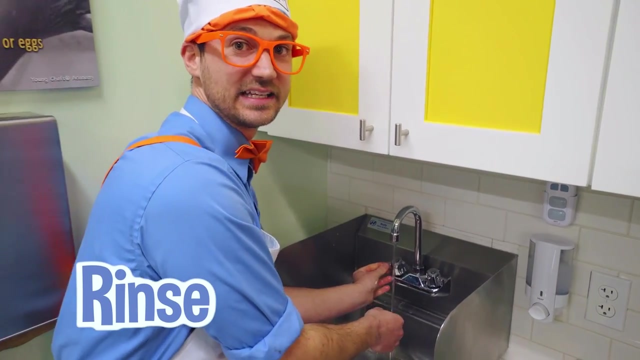 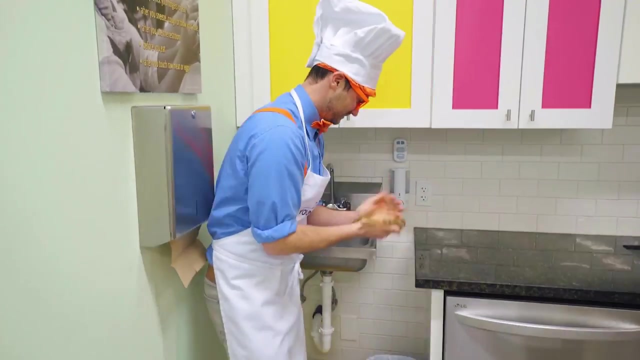 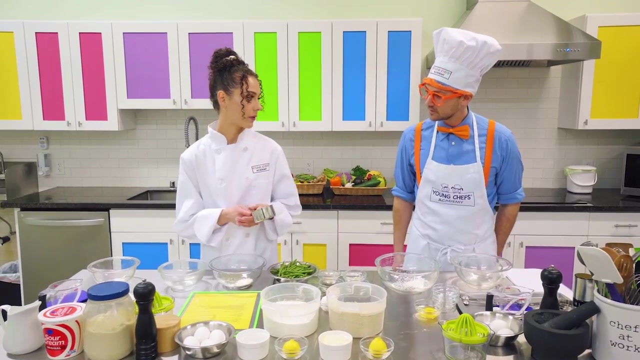 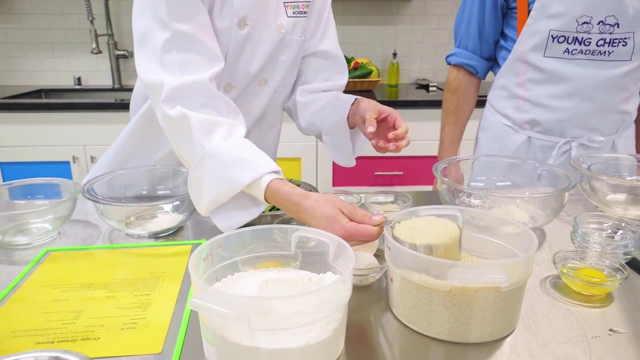 all right, there we go. let's rinse them off. it's really important to rinse off your hands and wash them completely after touching raw eggs or meat or anything like that. now we're ready, okay, all right. next we're gonna want to do a cup of panko, okay, so that looks about right. yeah, it's just panko, just like breadcrumbs. 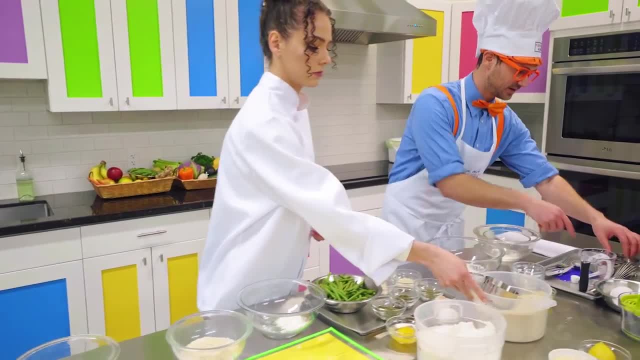 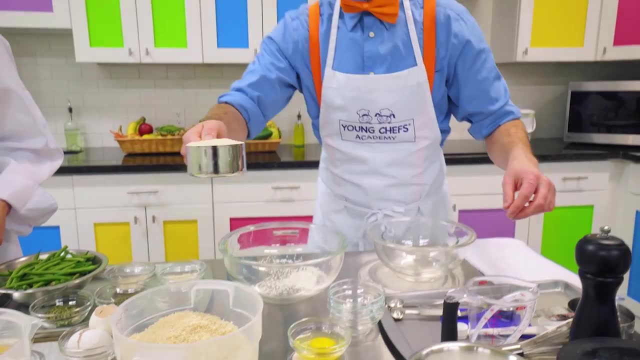 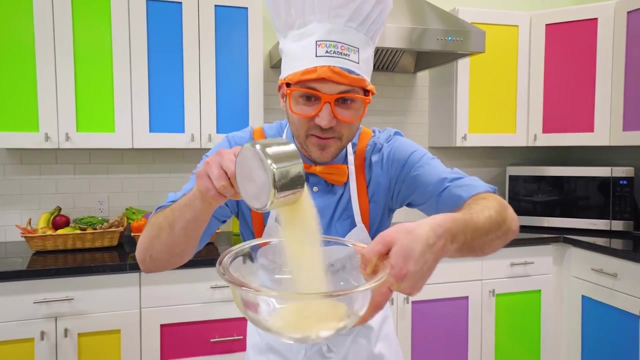 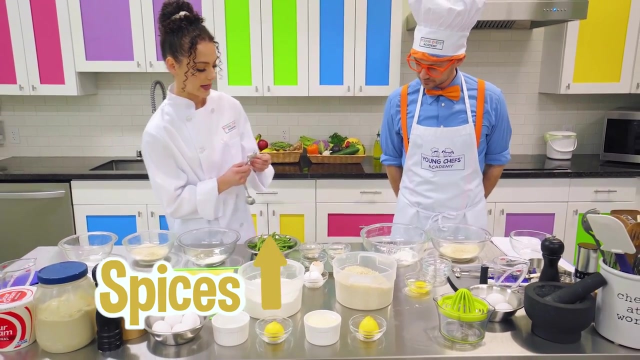 it is dried bread from. okay, all right. oh, let's use that. okay, one big scoop, all right, in the same bowl. yeah, oh, so sorry, in a different bowl. okay, oh, thank you. okay, here we go. weee, perfect, all right. next we're gonna want to add the rest of our spices, which is garlic salt. 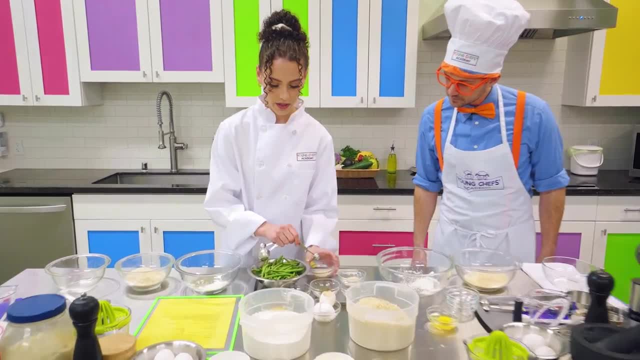 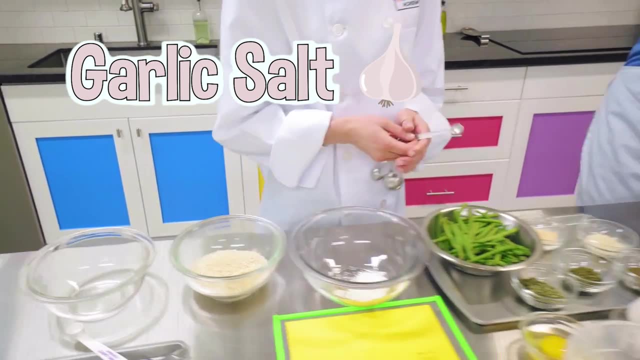 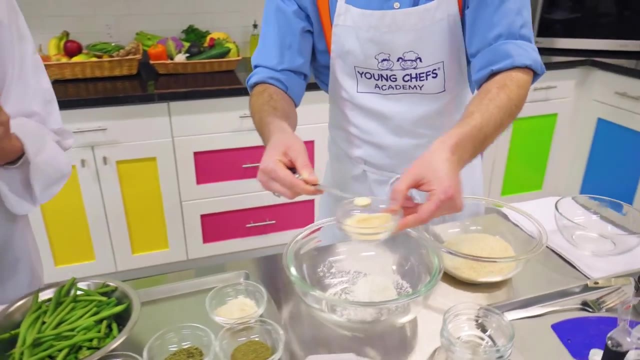 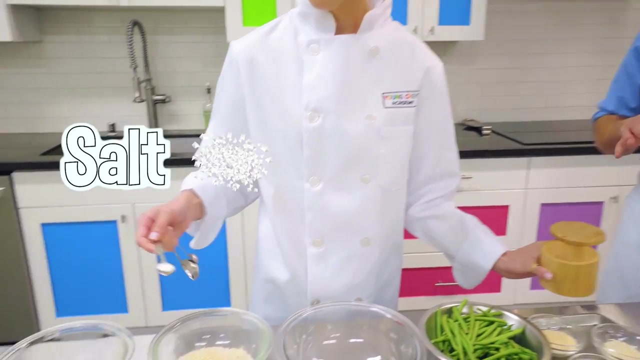 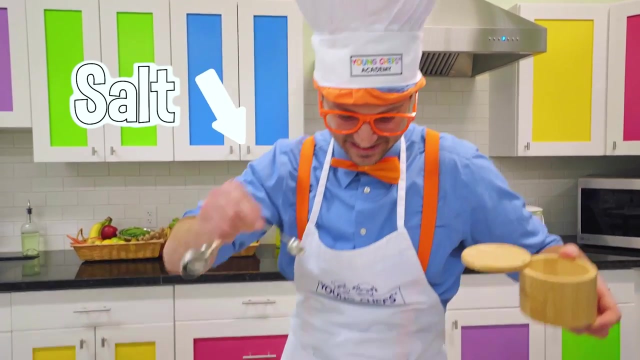 and salt. okay, so we're gonna want to use a tea, a fourth of a teaspoon of garlic salt in our panko. there we go. this one, okay, then put it in the panko, perfect. and then half of a teaspoon of salt, thank you, wow, salt is so yummy. here we go. can you use your whisk and whisk that up? 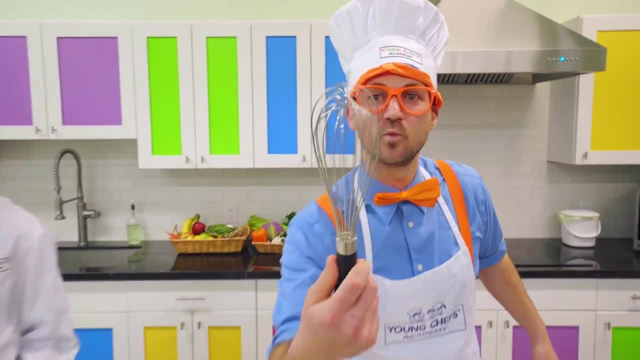 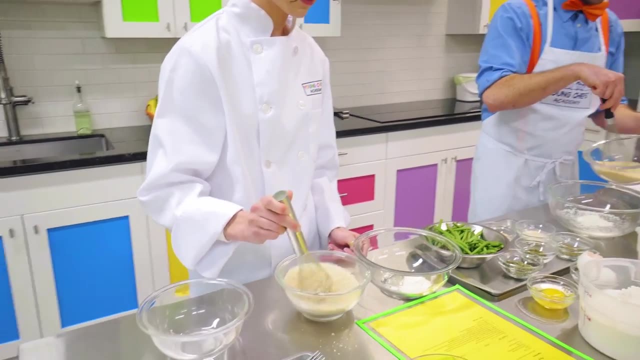 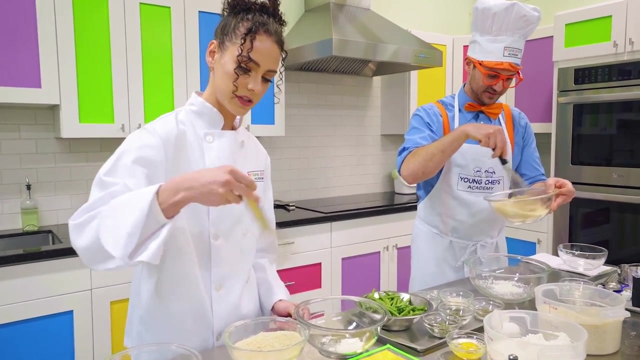 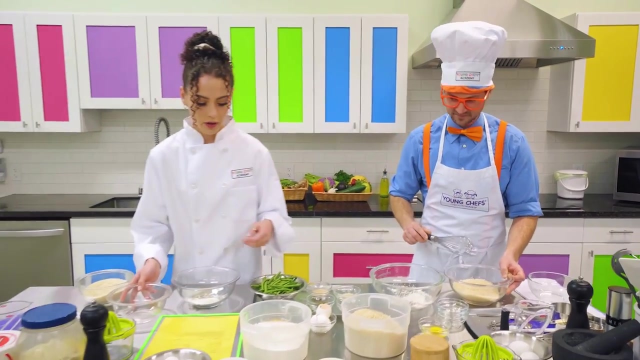 yeah, check it out. this is a whisk. yeah, how do you do it? whisk with your wrist, okay, oh, this is a really good way to mix it all up. yeah, you want to use it like that, all right. next we're going to want to put our egg into this mixing bowl. 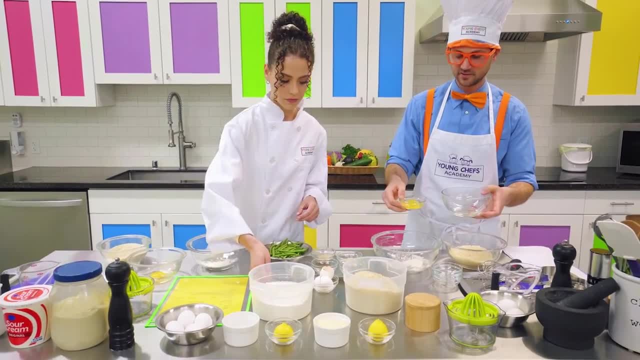 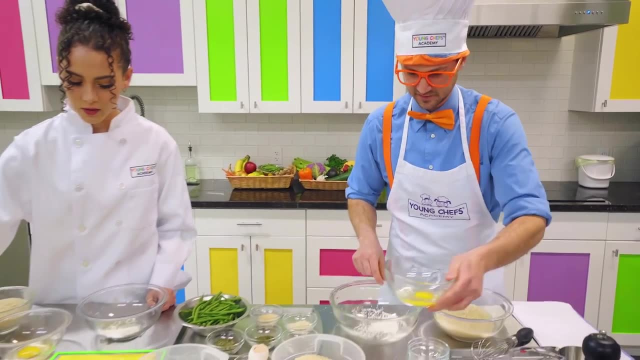 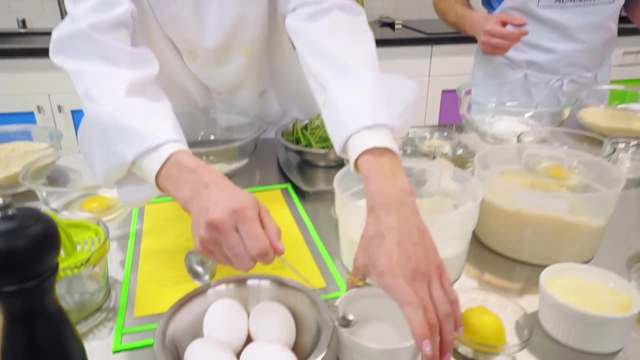 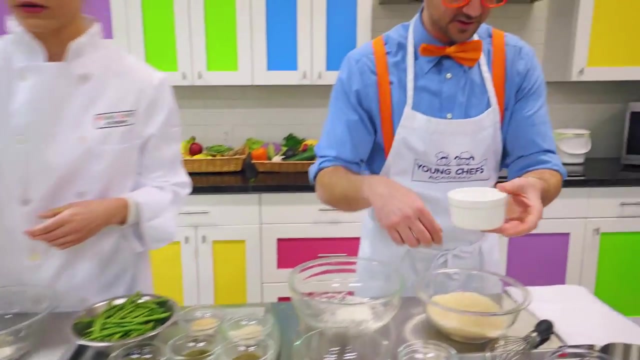 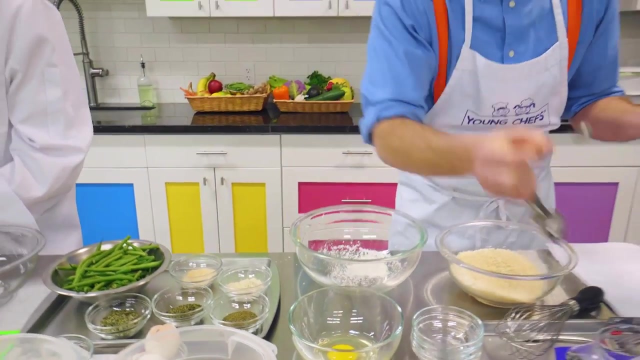 the clean mixing bowl that we have. okay, here we go, put the egg in this bowl, all right, and we're going to want to use a little bit of water? all right, just a little bit of water like this in the egg. perfect, thank you. all right, get some water in with the egg. perfect, can you whisk that? 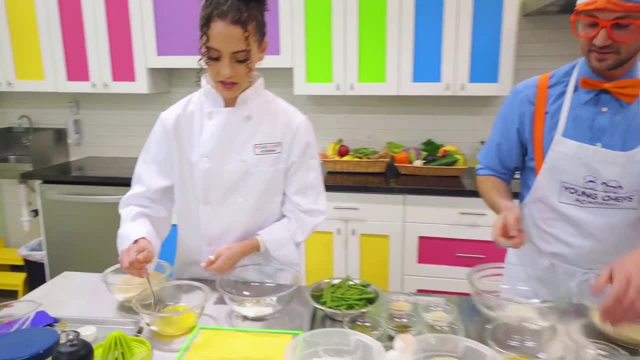 egg up with the fork. for me, with the pork, the forks are easier to whisk eggs and whisk is: oh, you want to whisk it first, like that. okay, so let's take them out of the Klari lid and put them in a bowl that we just made a sieve, just kind of for me to weigh in. so we don't want our sauce long slices. while we're cooking this inside the pan. so we don't want that gotten quick, so let's get them back into the pan. we have just kept this a good chunk, but we put that in it with us and then we we'll add the rest to the man and then afterwards we're going to add three comes right now, so I'm sending it to the man. 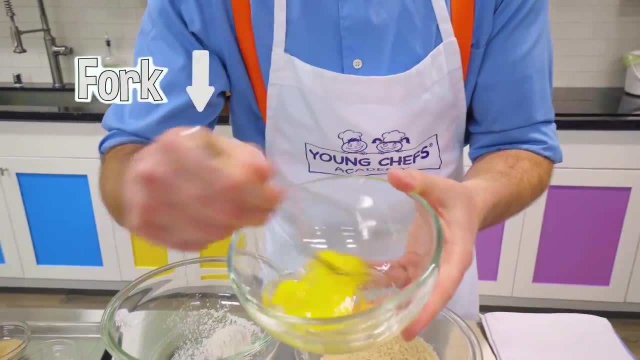 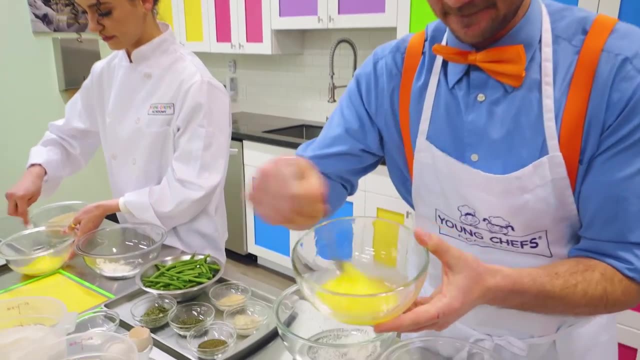 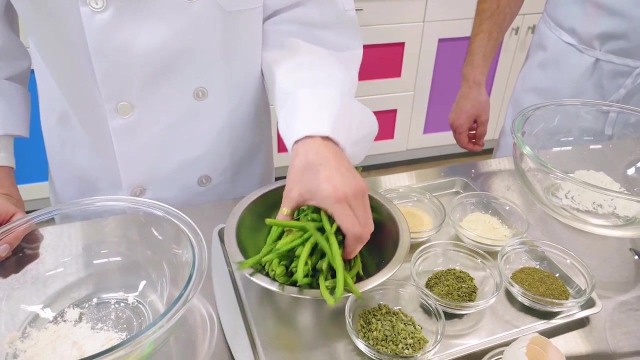 Okay, so let's take the fork and let's whisk the egg. Whoa, did you see how the yolk broke up? And now it's all mixed up. Perfect, That's perfect. We're gonna grab a couple of handfuls of green beans. 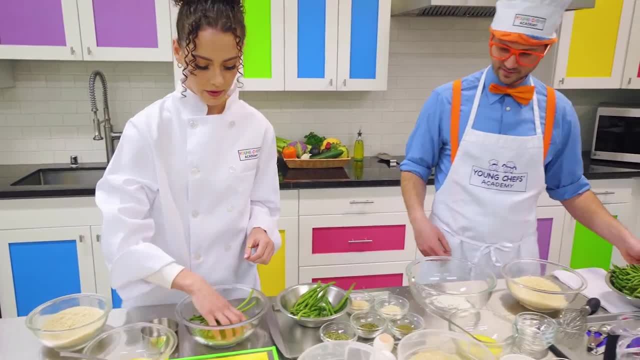 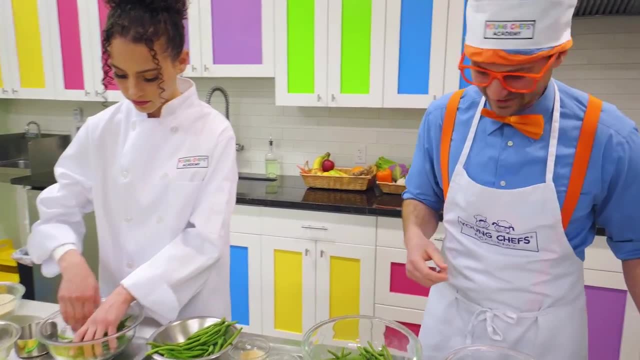 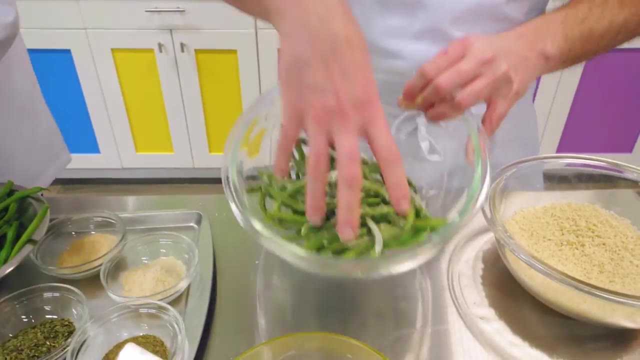 right in here. okay, right, perfect, And toss it in our flour. All right, Make sure you get them all nice and mixed up and coated in flour. Okay, toss it. Wow, This is gonna help the egg stick to the green bean. 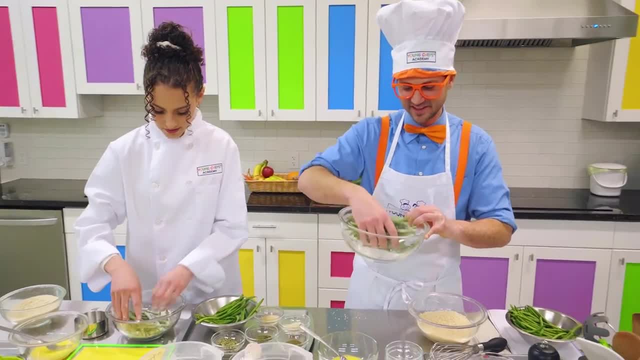 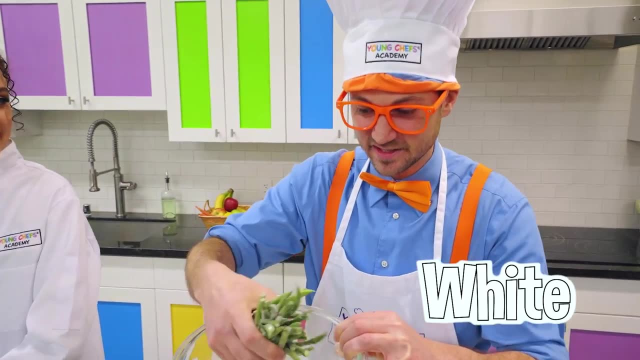 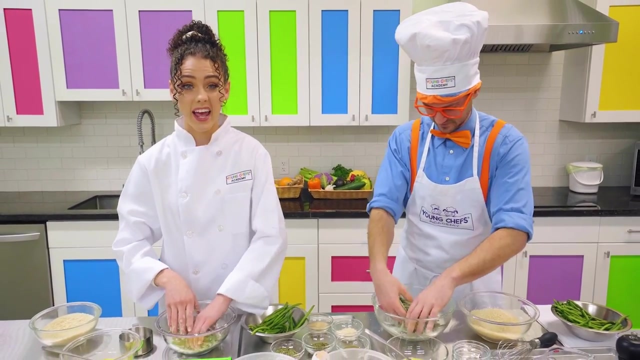 Okay, interesting. Look, they used to be green, but now they're green and white. Hey, remember how we washed our hands? Yeah, good thing we did, because I'm touching food with my hands. You don't wanna touch anything after you touch egg or raw meat. 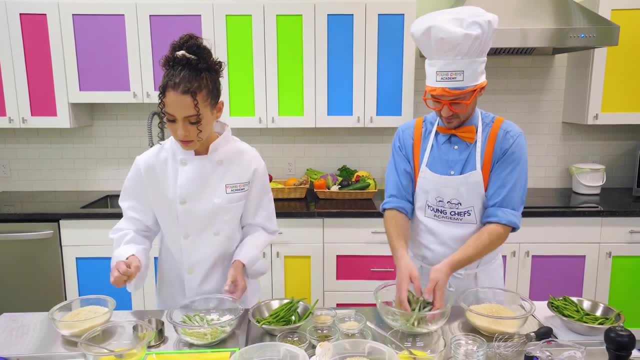 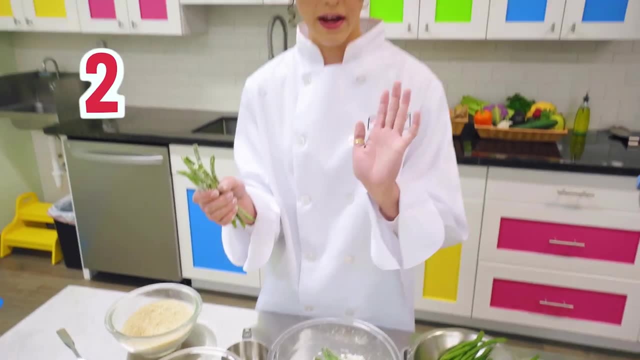 So you wanna make sure you wash your hands? Okay, All right. now we are gonna touch the egg, We're gonna put the green beans. We're gonna use two different hands. We're gonna have our dry hand and our wet hand. 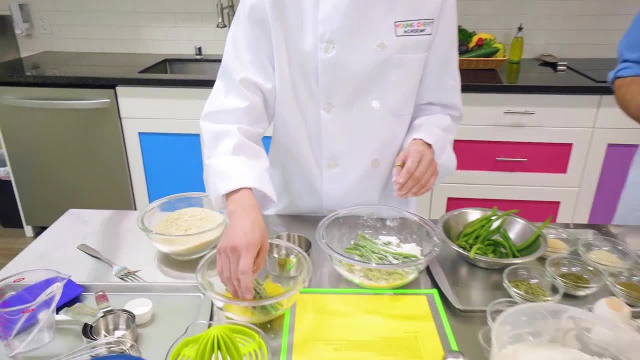 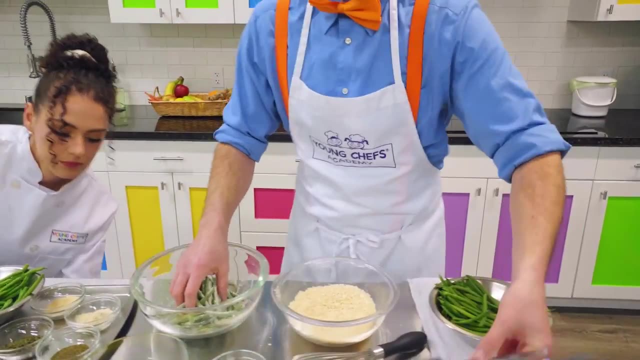 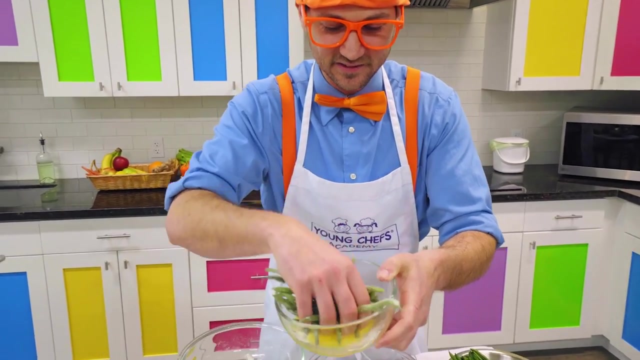 So we're not gonna touch the egg with this hand. We're gonna put our green beans in here and toss it around. Okay, take the fork out Now, let's do a little tossing. There we go. Whoa, I'm spilling. 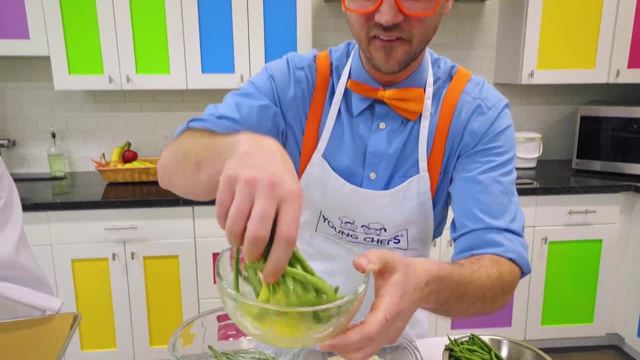 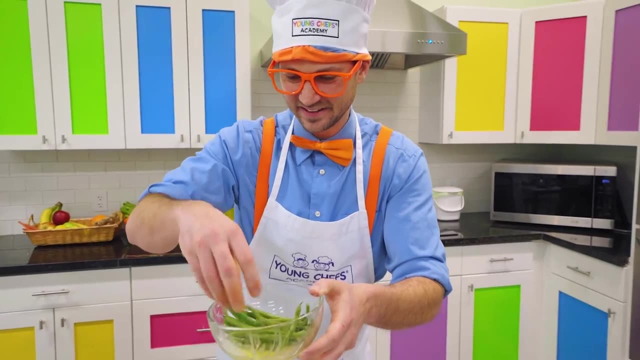 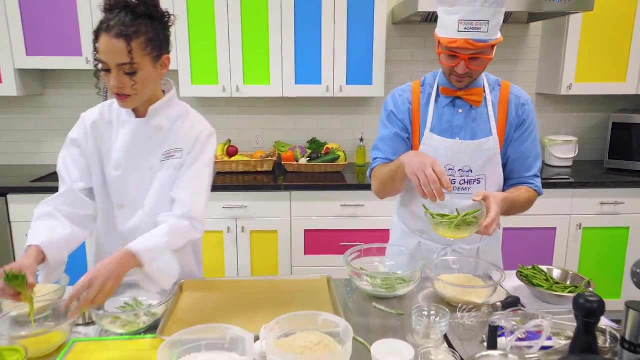 That's okay. Okay, wow, Look at it. There's so much egg on these green beans. Okay, All right. great, Now you're gonna wanna put the green beans into the Panko, Toss them around real quick, Okay. 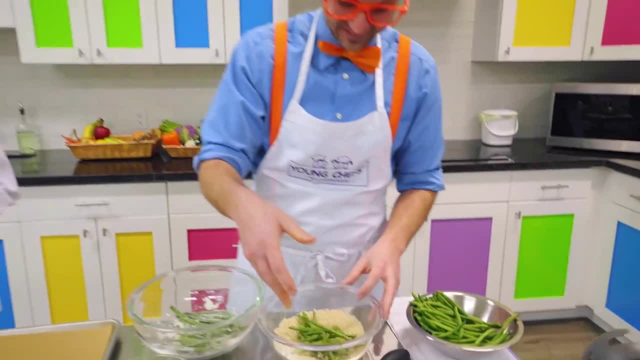 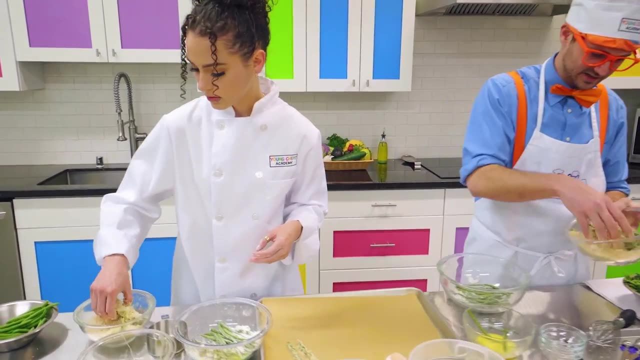 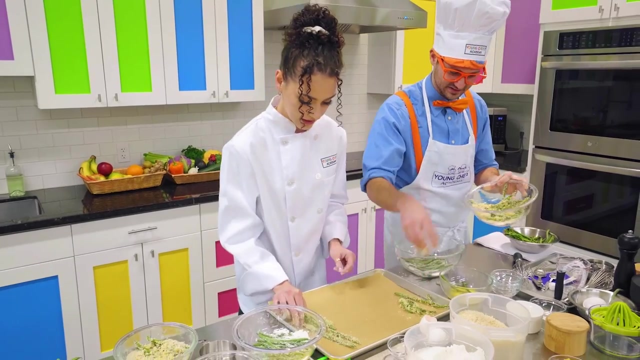 Wow, Good job. That looks fun. And once they're nice and evenly coated in Panko, you wanna put them onto the tray. Okay, These are gonna be so yummy. I know I'm excited. Let's put them a little bit nicer. 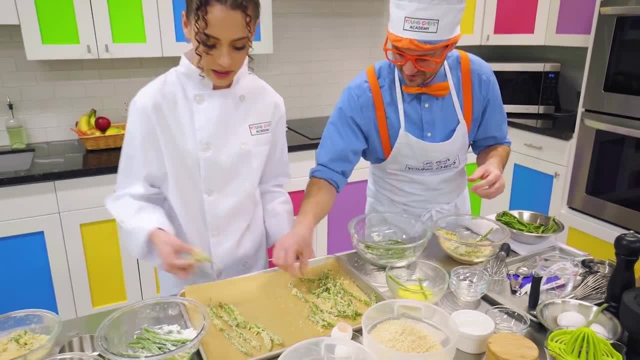 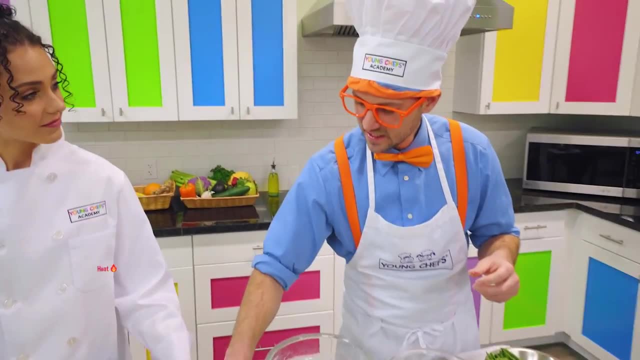 so that they're not so messy. Okay, That way they'll cook really evenly when they're spread out on the tray. There we go. That makes sense. Oh, I see, Because if they're on top of each other then the heat can't touch the whole green bean. huh. 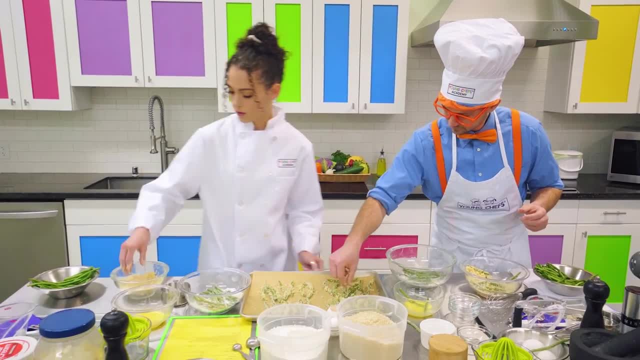 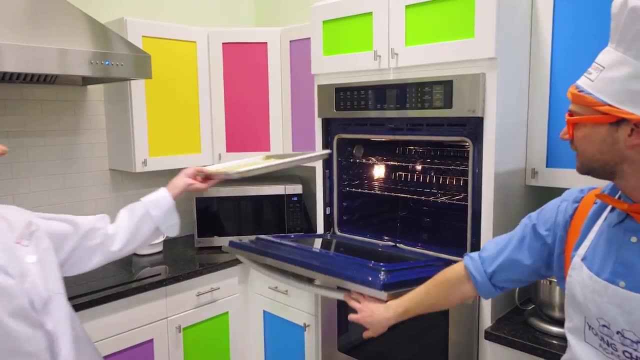 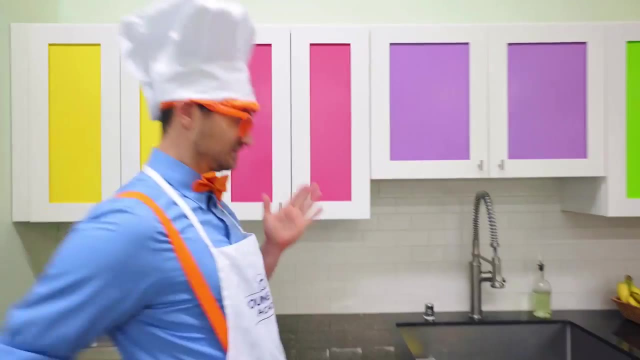 Exactly. You wanna make sure that the whole thing is getting cooked. We're ready for the oven. Okay, here we go, Here you go. Thank you, Perfect. Those will take about 10 to 12 minutes to cook Whoa. 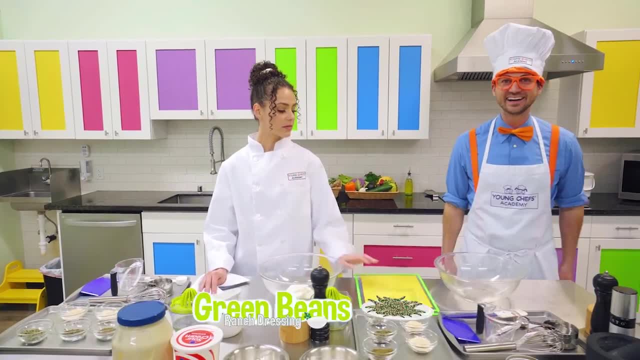 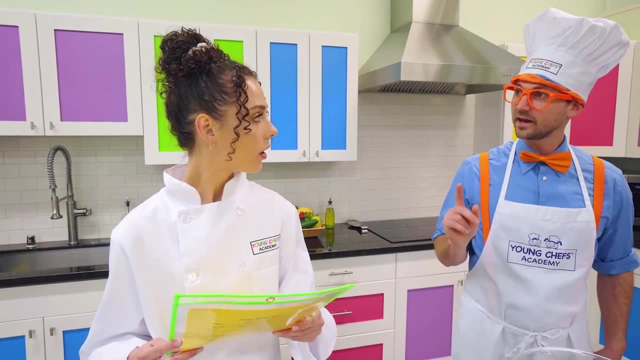 That was really fun making those green beans with you, Wasn't it? Yeah, let's make some ranch the peppermint. What ingredients do we need? We need mayonnaise, sour cream, buttermilk. Wait, did you say buttermilk? Yeah, Oh, I said cream earlier. 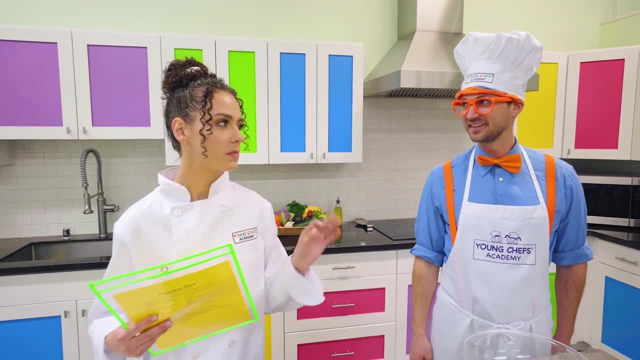 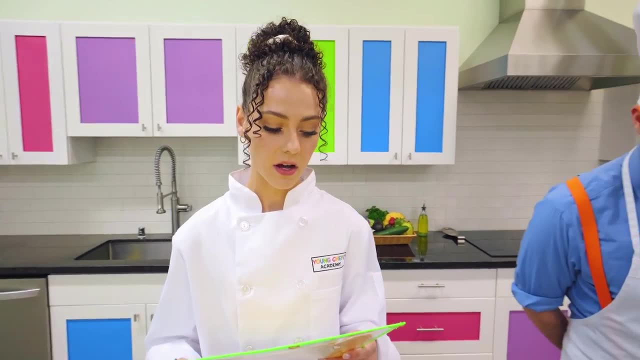 Okay, so we need buttermilk. Yes, they're very similar, but buttermilk smells different and it's a little thicker. Okay, All right. lemon juice, dill, weed, parsley, chives, onion powder, garlic powder. 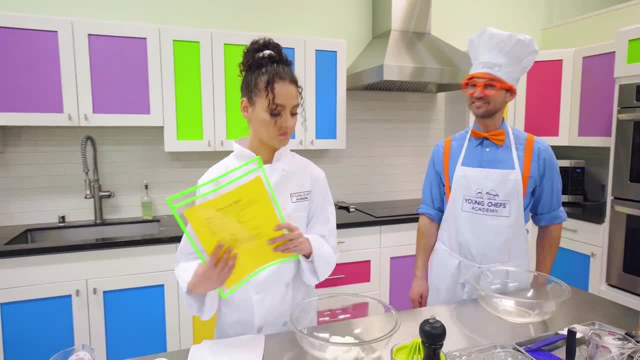 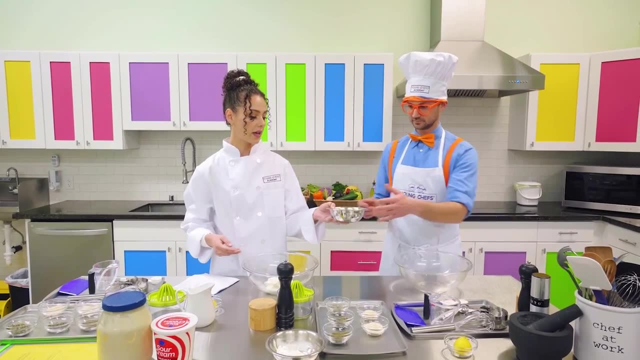 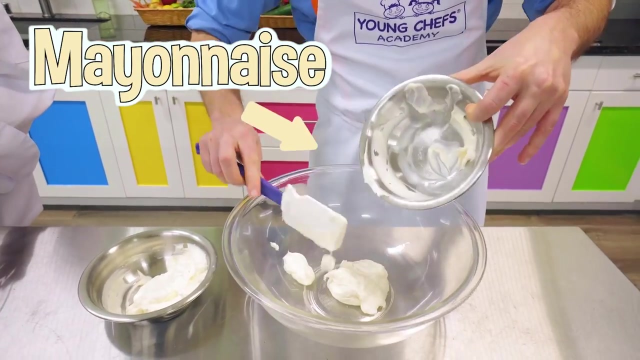 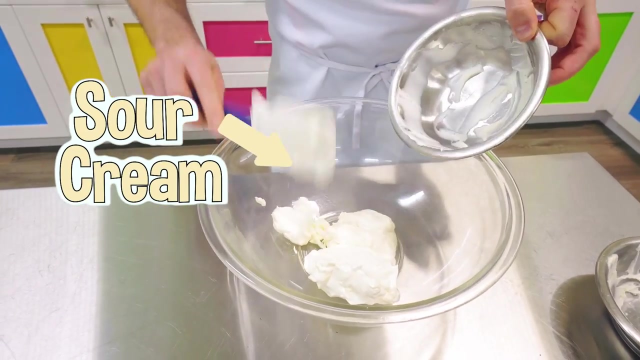 salt and black pepper. Okay, perfect, Looks like we have everything I think we do. All right, next we're gonna wanna, So I have mine all mixed up. Can you put the mayo and the sour cream into your big bowl? Okay, here's the mayo, Then we have the sour cream. All right, there we go. Awesome Now. 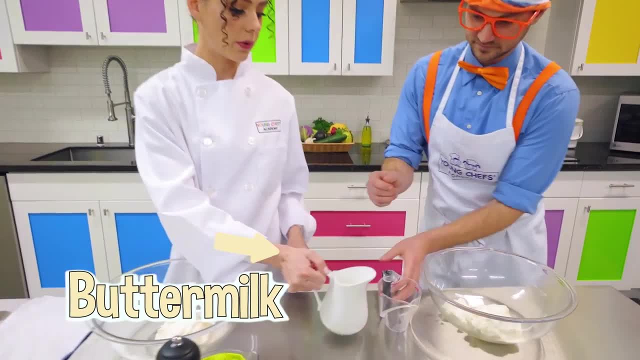 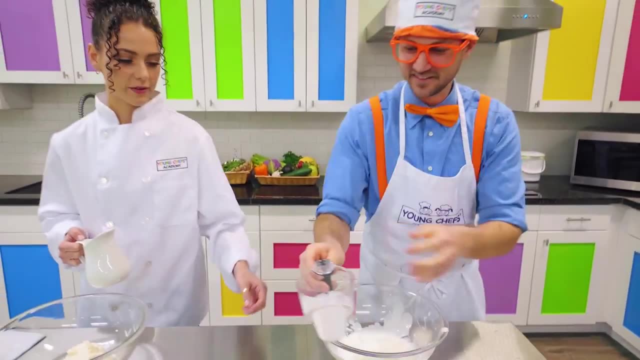 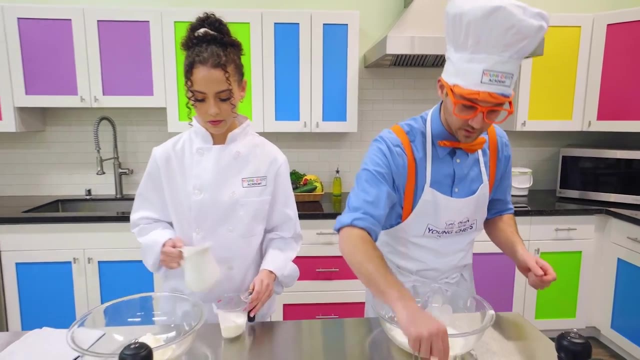 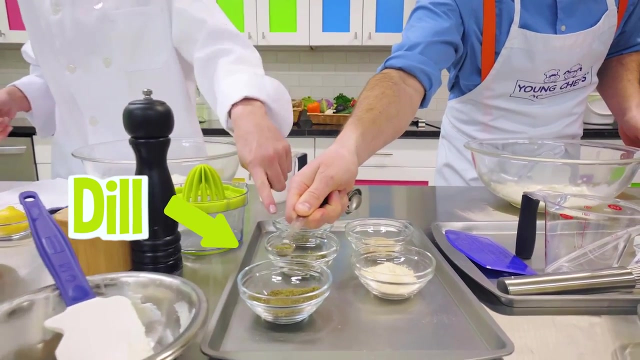 we're going to want to do half a cup of buttermilk into your bowl, All righty, There we go, Perfect, All right. now we're going to want to get our one-fourth teaspoon- Okay, perfect, I'm ready, And we're going to use that for our dill right here. Okay, Parsley. 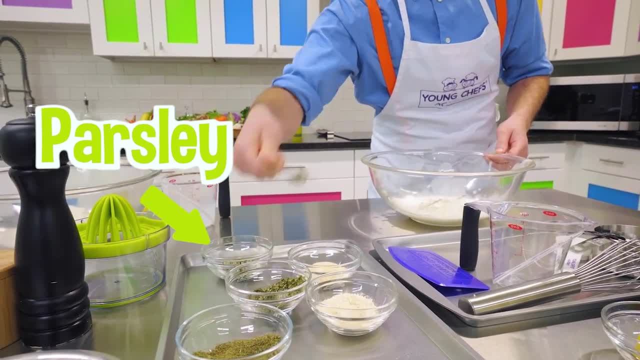 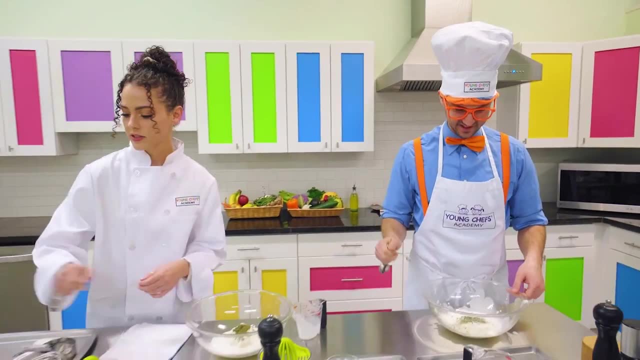 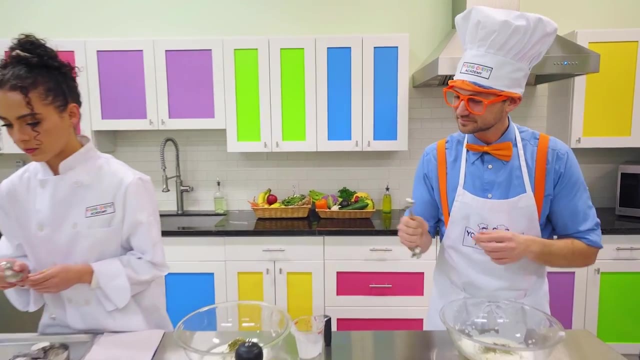 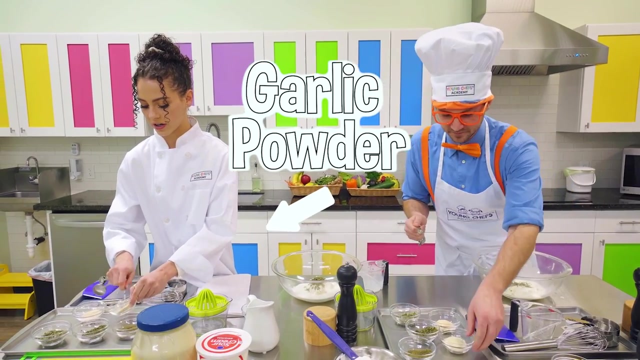 and our chives. Okay, dill parsley and chives. There we go. Good job, puppy. Next we're going to want our half teaspoon- Okay, A little bigger, All right. All right, and we use that for our garlic powder and our onion powder, All right. 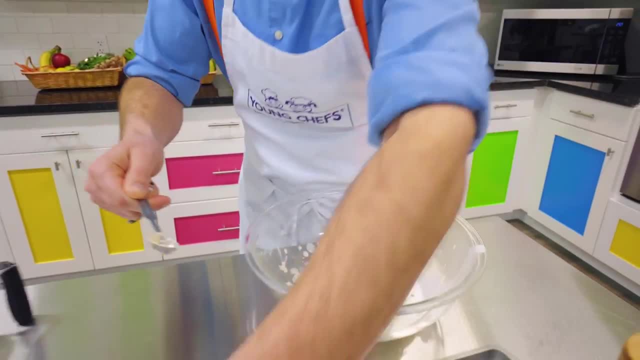 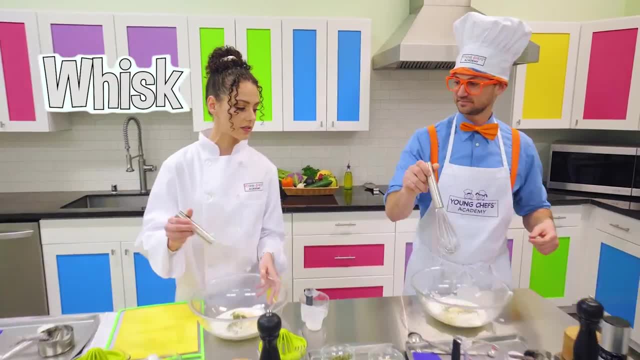 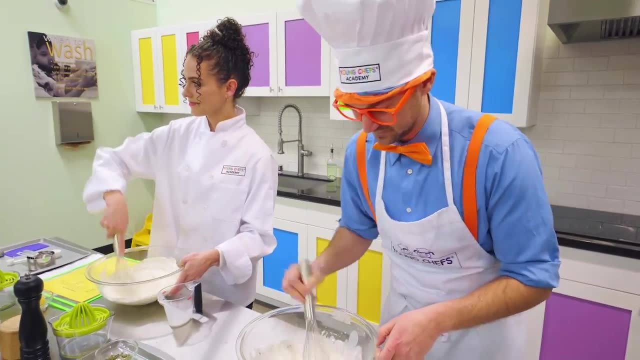 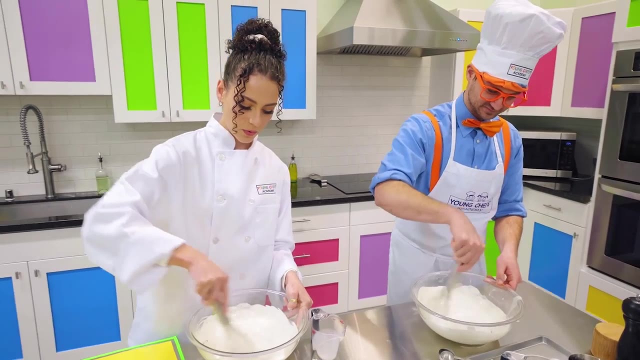 Let's mix that up with our whisk, And don't forget, we whisk with our wrist. All right, Whoa, this smells so good. Once it's all mixed up, we're going to cover it and place it in the fridge to cool. 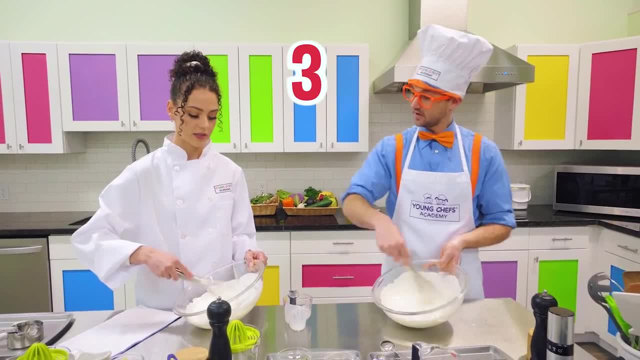 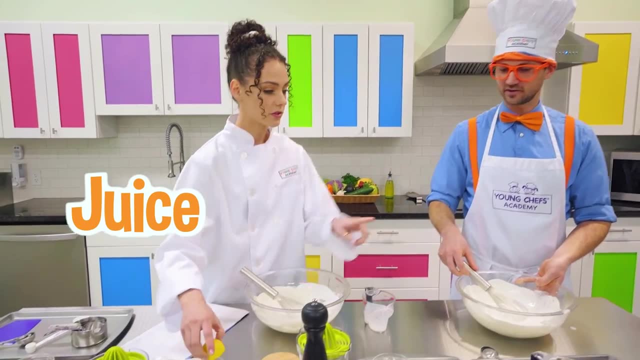 All right, We only have three more ingredients. Okay, what are they? Lemon juice, salt and pepper. Okay, First we want to juice our lemon. So you have a lemon right up there, Perfect, We have it cut in half and we'll use our juicer here. We want to make sure we 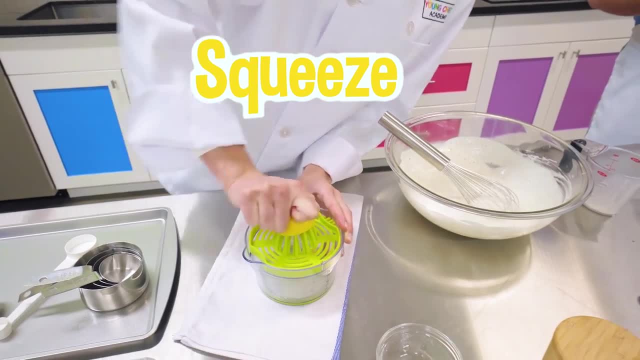 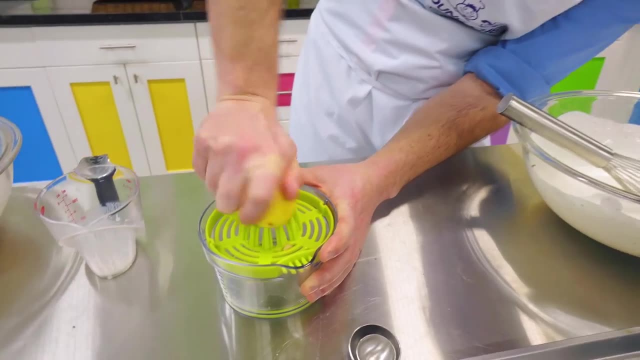 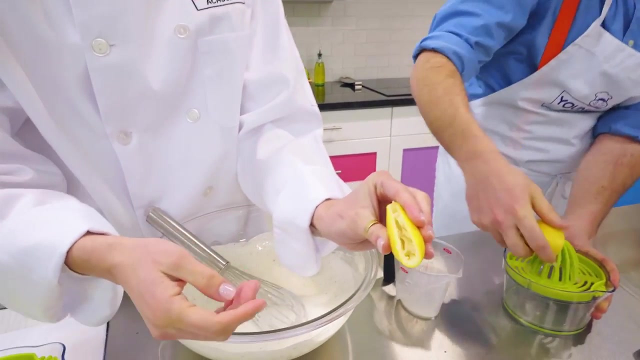 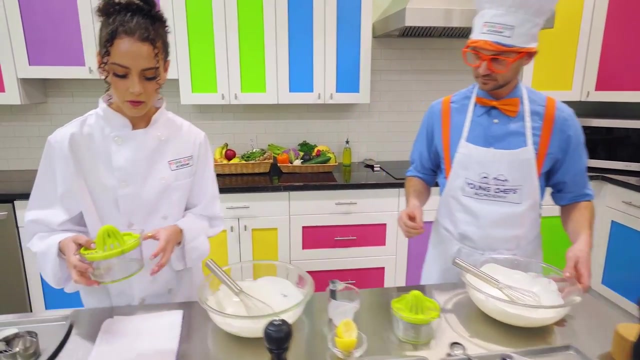 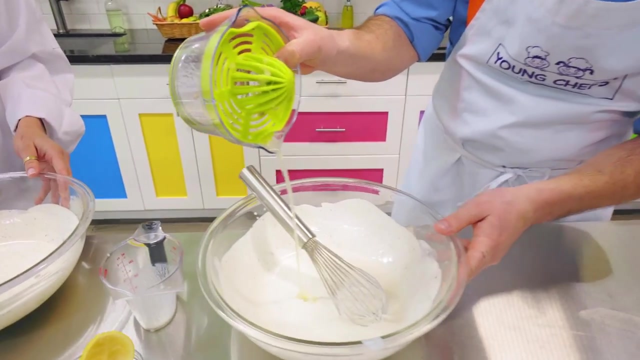 squeeze really tight, pushing down and twisting it around to get all of that juice out. Okay, I guess I'll try it. There we go. Good job, Yeah. When you take it off, your lemon should look something like this: Yeah, It's almost empty. Perfect, Good job, Okay. And then we want to pour our lemon juice into our ranch. Okay, Here we go. Whee, Awesome, Mix that up. 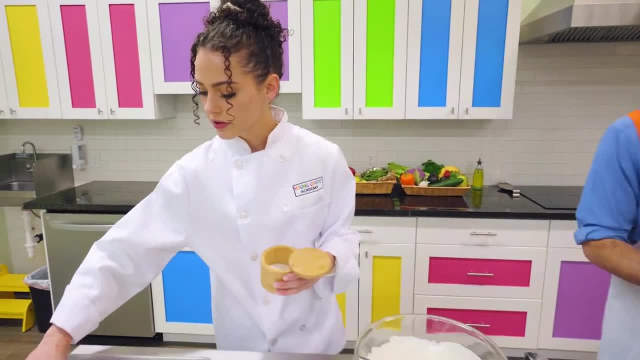 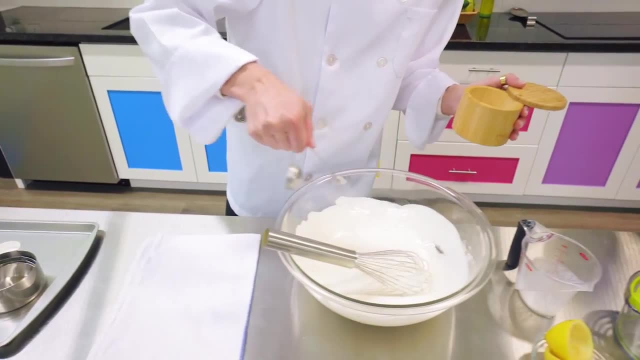 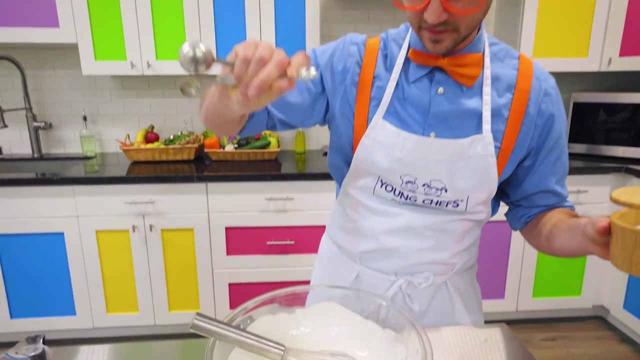 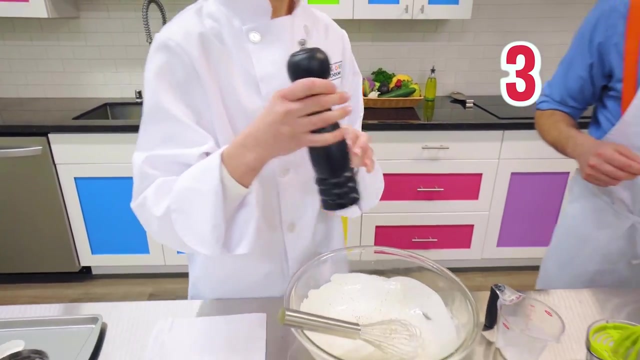 All right, Now we want to do one-fourth teaspoon of salt Right like this: Okay, Put some salt in here, There we go, And a pinch of pepper. So we'll go about three twists. Okay, One, two, three, Perfect. 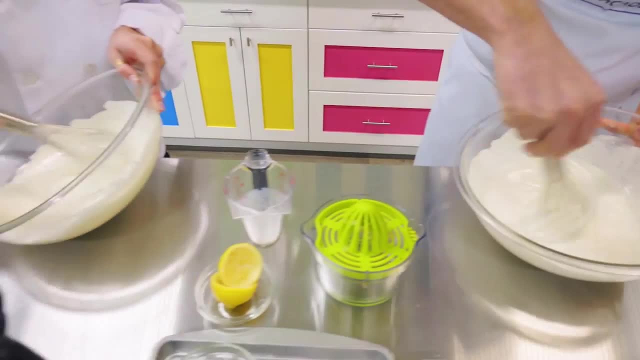 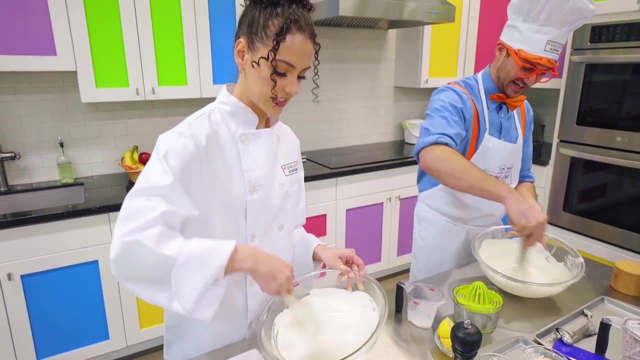 All right, Let's mix that up. All right, Mix, mix, mix. Remember to mix with your wrist. Oh yep, Oh wow, this is going to be so yummy, Delicious. Did you hear that? I did. 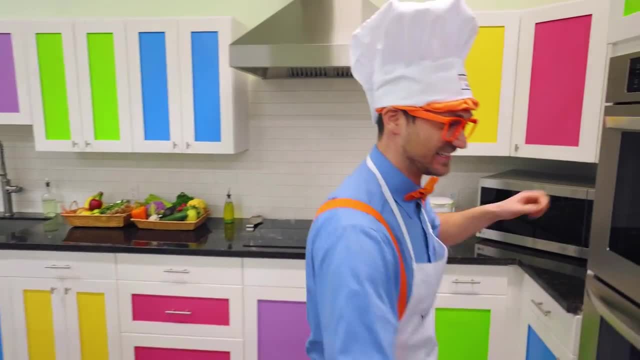 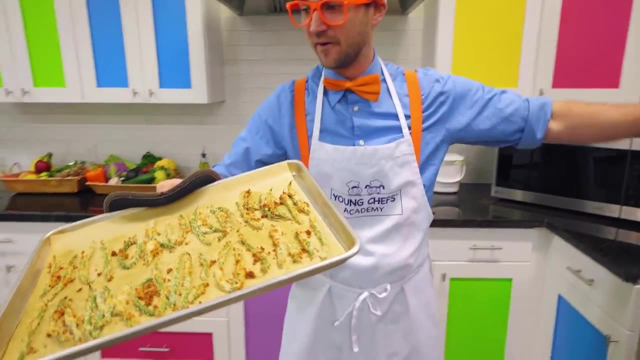 Does that mean the green beans are done? It? does you want to grab them? Sure, Oh, this is going to be awesome. Oh, yum Wow, Those look delicious. Blippi, Wow, check them out. Oh my gosh. 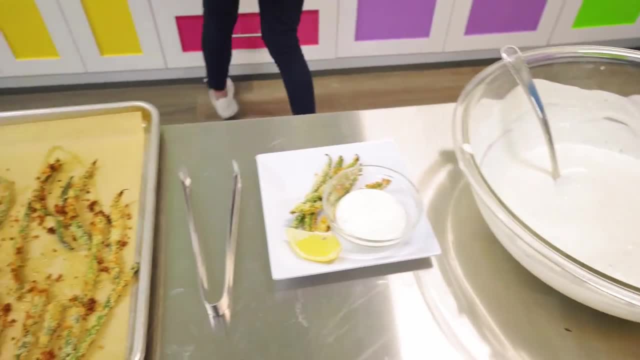 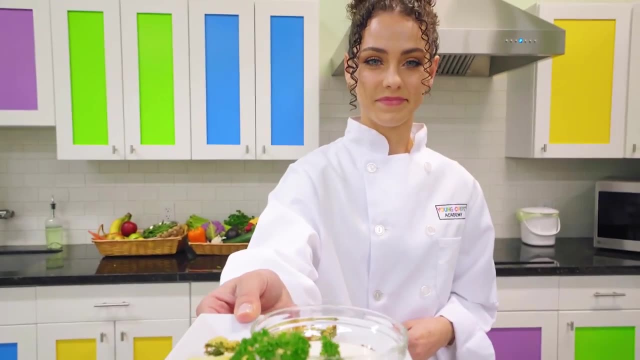 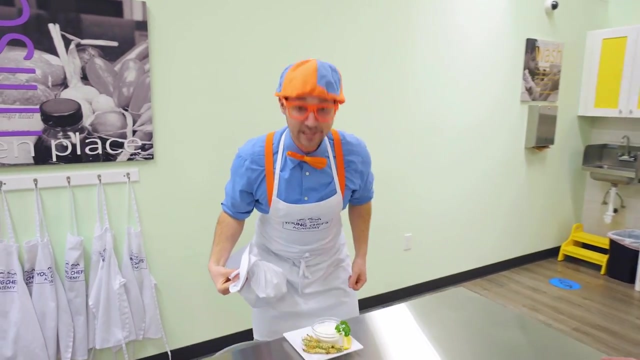 All right, Blippi, it looks like our green beans and zesty ranch are all ready. They look so good. Those look yummy. Check them out. Whoa, I am so excited. Thank you so much for teaching us how to make these. 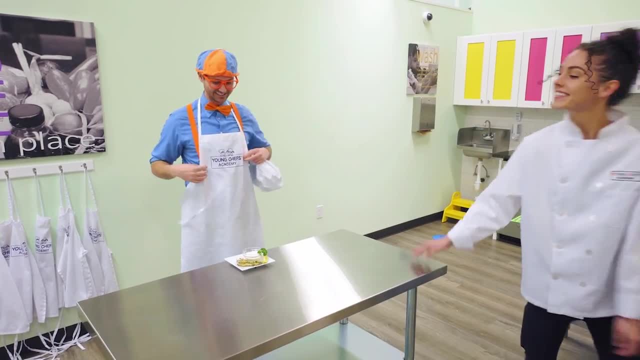 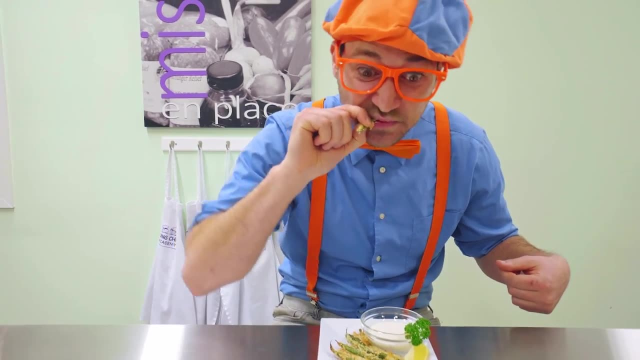 Of course you did such a good job. Come back every time, Oh well, thank you, See you later. See ya, Wow, I am so excited, Here we go. Yum, That is zippalicious, So silly.